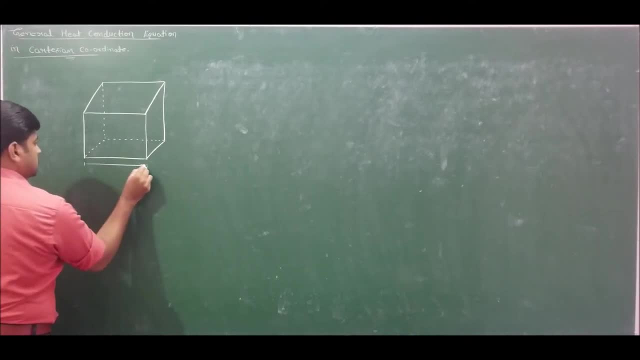 the volume of this element be dx, dy and dz. like there is a heat conducted to the system around x axis, be qx, and heat leaving in the x direction be q of x plus dx. Similarly, heat entering this volume in y direction be qy, whereas heat leaving this volume in y direction. 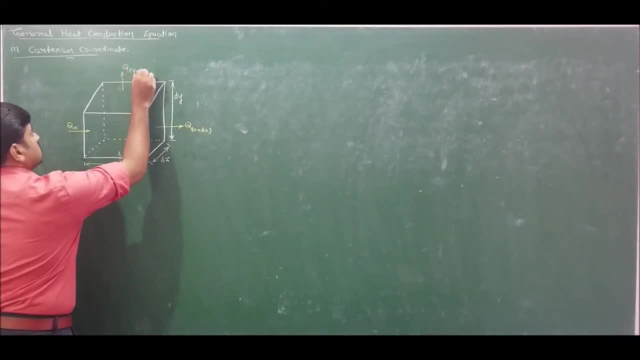 be q of y plus dx. Similarly, heat entering this volume in z direction be qz, and heat leaving in z direction be q of z plus dz. Now let me place this in a Cartesian coordinate system like this: Let this be x axis and this be y axis, sorry, z axis and this be y axis. So we are considering: 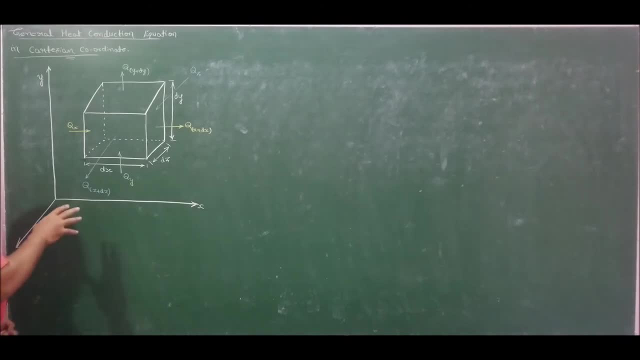 an elemental volume, as shown in the figure, wherein which the heat entering the volume be qx in x direction and leaving is qx plus delta x. Similarly, I wrote the entering and leaving of heat in all the three directions, in addition to which there will be an internal. 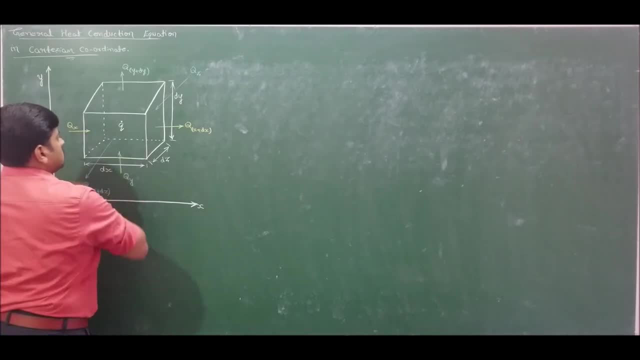 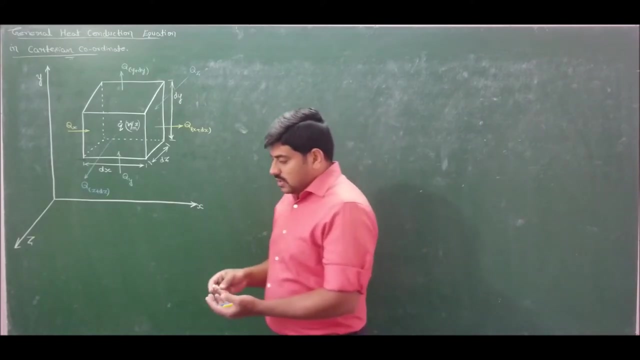 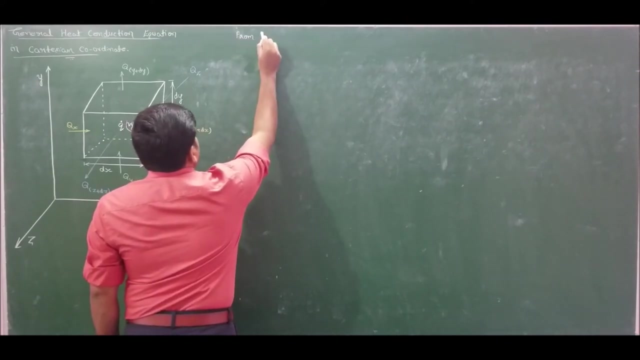 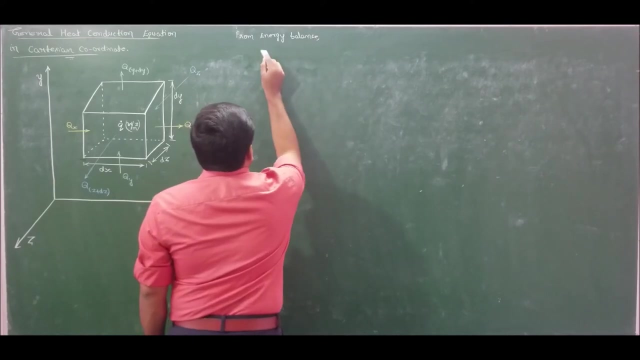 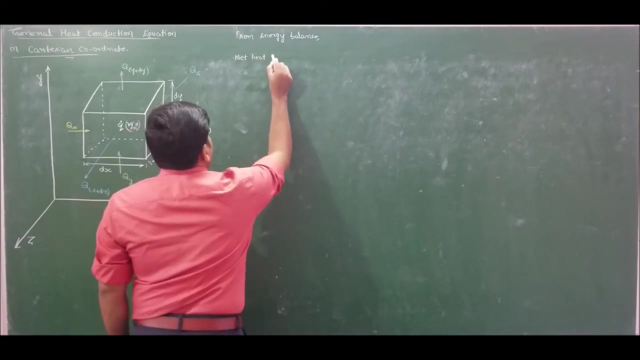 heat generation of q dot Watt per meter cube, in addition to which we are considering an internal heat generation of q dot Watt per meter cube inside this volume. Now, if I write energy balance to this system, So from energy balance I can write net heat conducted into the volume per unit time per. 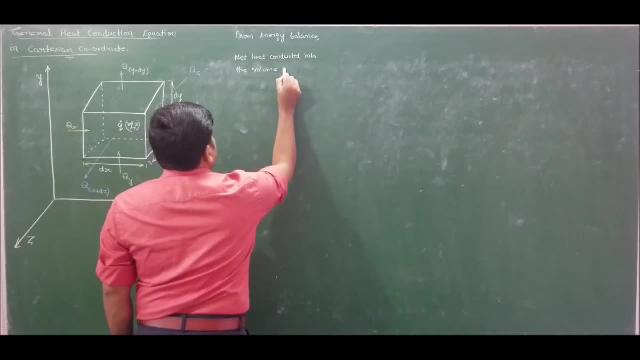 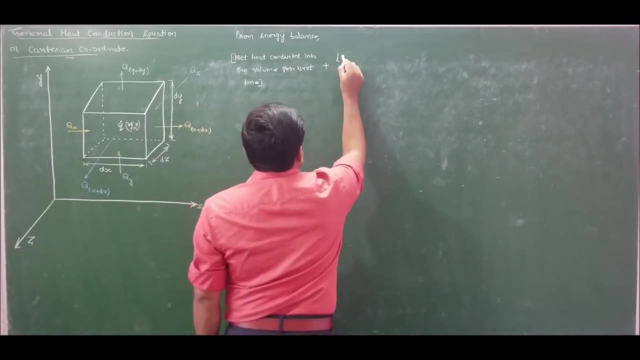 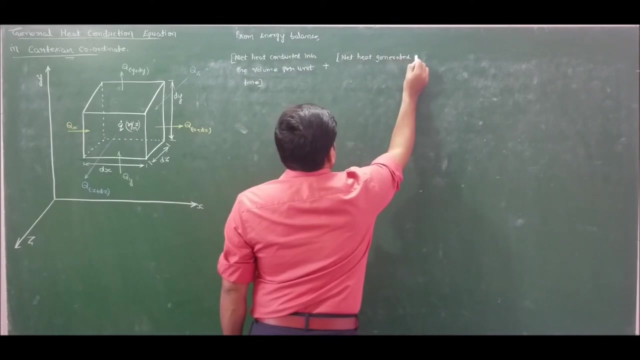 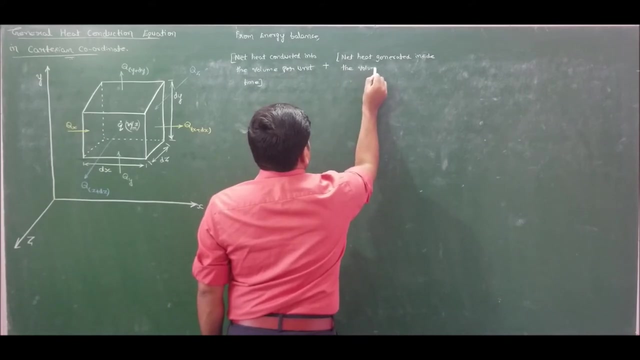 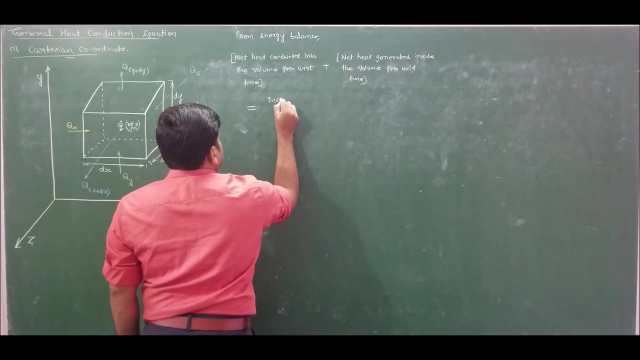 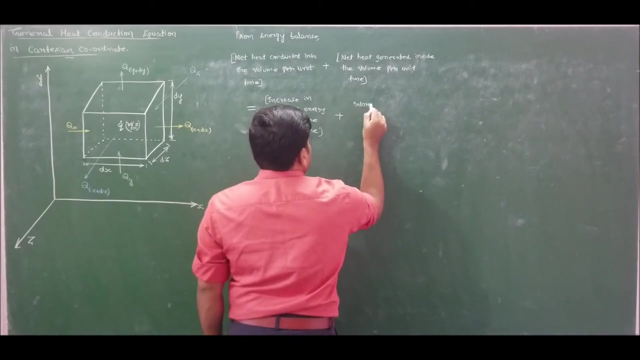 unit time. per unit time plus net heat generated inside the volume per unit time Must be equal to increase in internal energy of system, increase in internal energy of the volume per unit time plus work done by the volume per unit time. 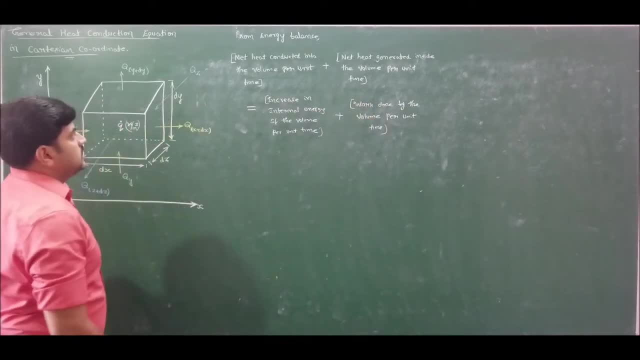 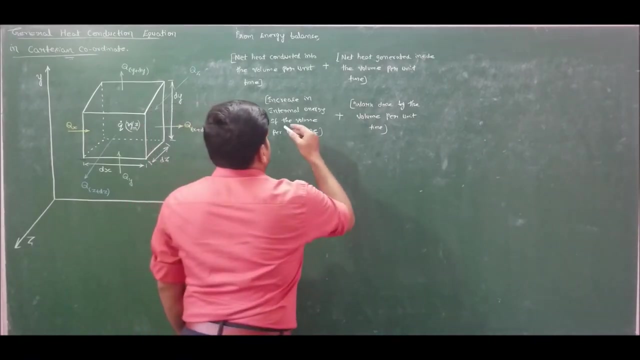 So if I write the energy balance for the system, net heat conducted into the volume per unit time plus net heat generated inside the volume per unit time, must be equal to increase in internal energy of the system plus work done by the system. Now let us take each term as. let us take this as term 1, this as term 2 and let me 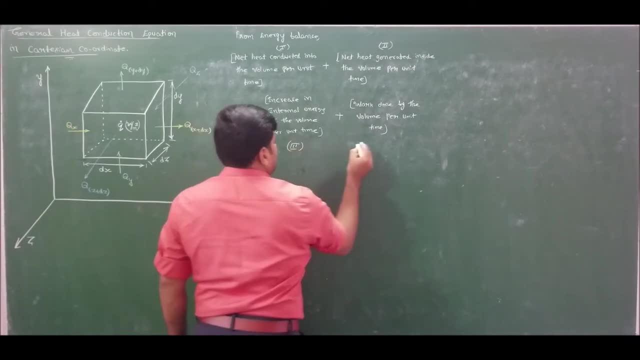 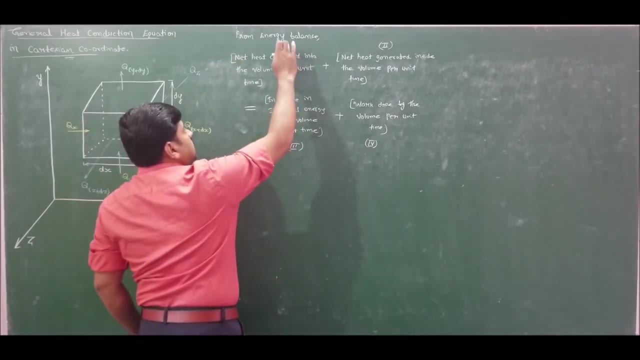 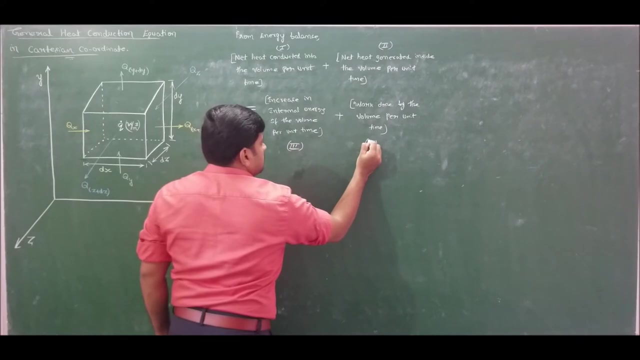 take this as term 3 and this as term 4.. Now, individually, I want to calculate the values of term 1, term 2, term 3 and term 4 and, substituting to this energy balance equation, I will get the general heat conduction equation. 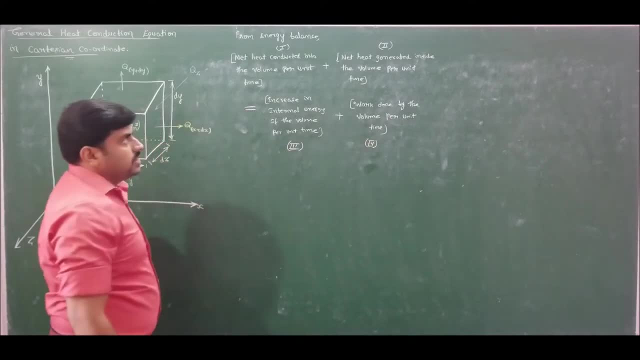 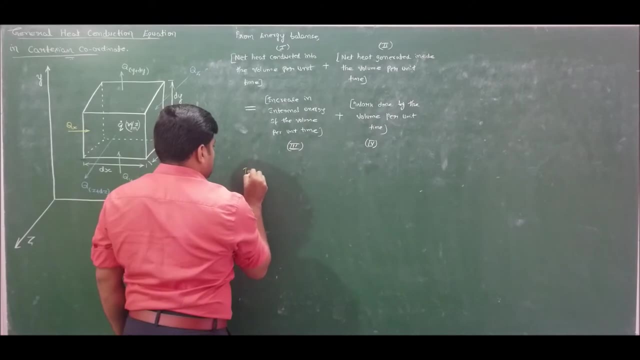 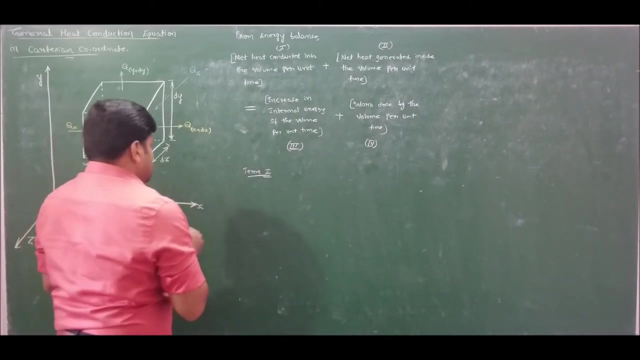 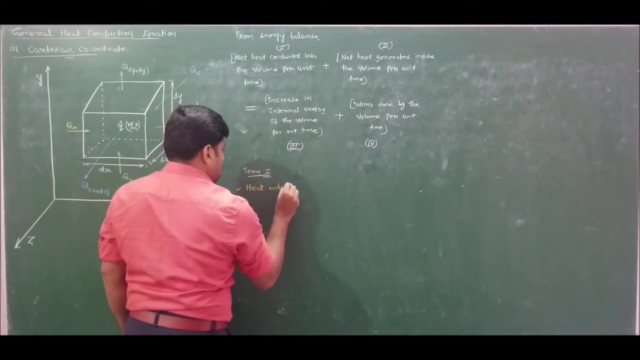 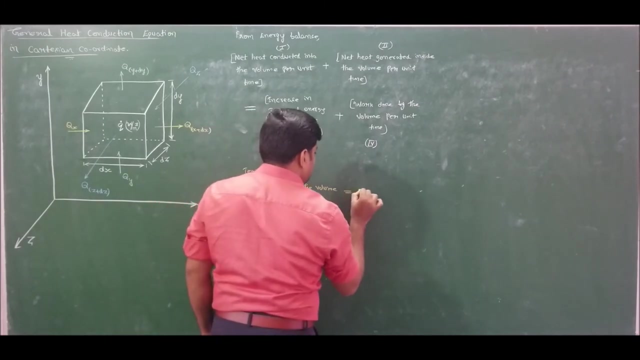 for the elemental volume shown in the figure in Cartesian coordinate system. Let us discuss one by one. if I take term 1, considering term 1,, so from the figure we observe that heat entering the volume per unit time is because of conduction. so therefore, 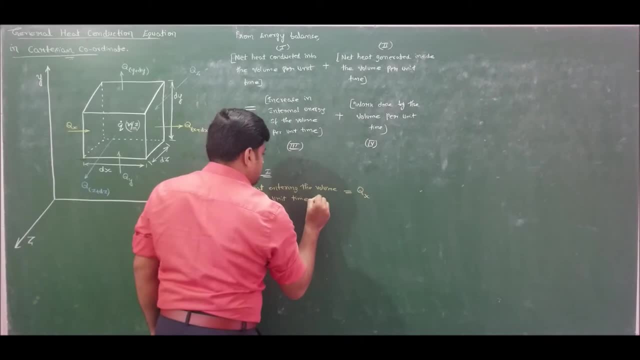 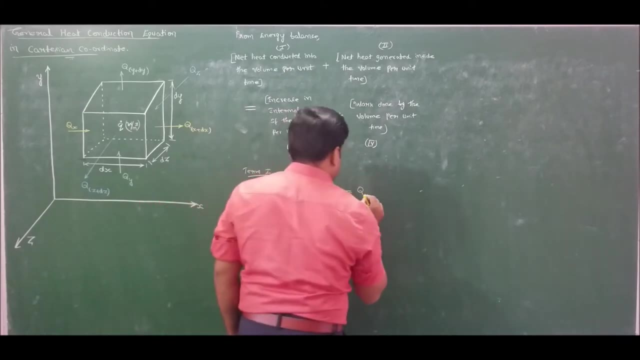 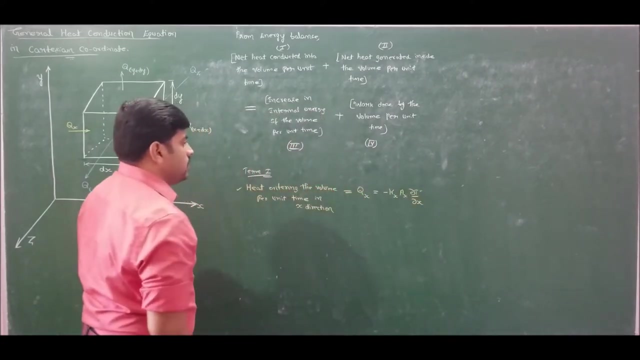 I can write it as qx in x direction. So I am going to write: qx in x direction is equal to qx, which is nothing but minus kx area along x direction, dou t by dou x. So I am using partial derivatives, because temperature is a function of space, that is. 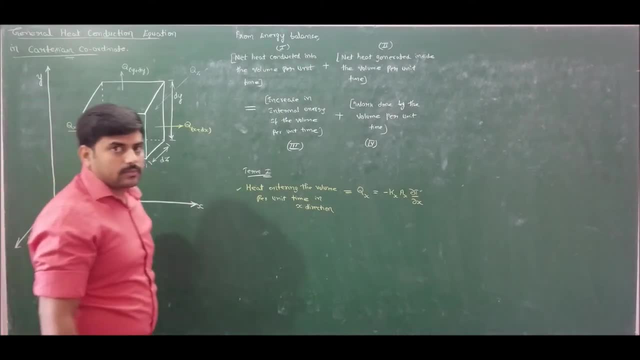 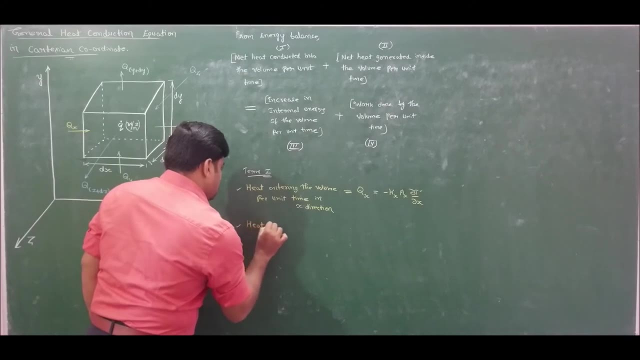 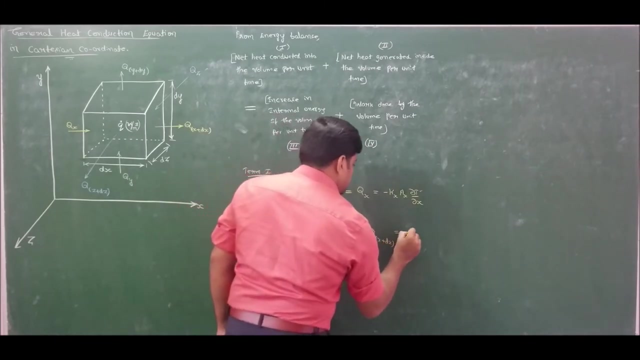 special coordinates, x, y and z, and also it is a function of time. So now, similarly, if I write heat, leaving the volume per unit time along x direction, is given by q of x plus dx, which can be written as qx plus dou, qx by dou x dx. 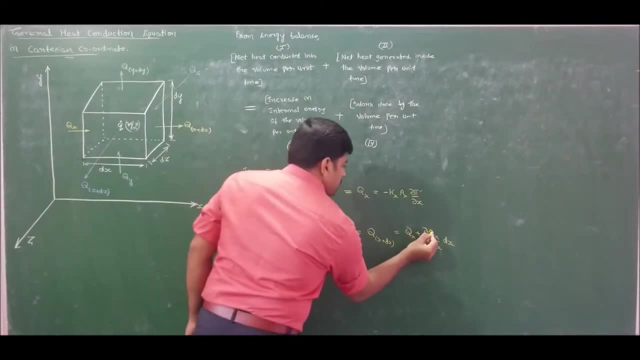 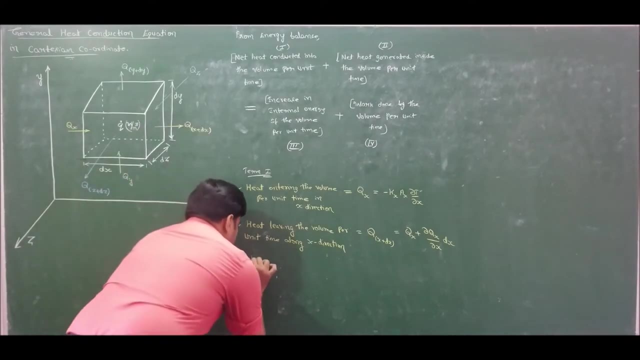 This you people already know. So now, if I calculate, the net heat accumulated along x direction will be net heat accumulated per unit time along x direction. along x direction will be, So qx is entering, whereas qx plus dx is leaving. So therefore net accumulation is what is entering. 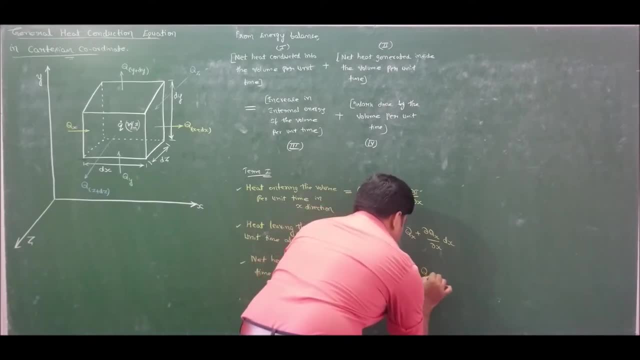 Entry minus. what is leaving Leaving is qx minus dou qx by dou x dx. So therefore I can cancel off qx and qx. So net heat accumulated will become substituted to the value of qx as kx area along x direction. dou t by dou x. I will get minus, of minus will become plus. 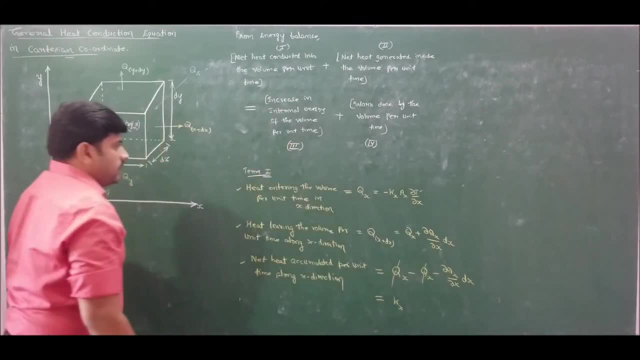 So I am getting minus of minus as minus. Now let us take a look at the equation of the thermal conductivity along x direction. Coming for area along x direction, I should take area perpendicular to the direction of heat flow according to Fourier law of conduction. 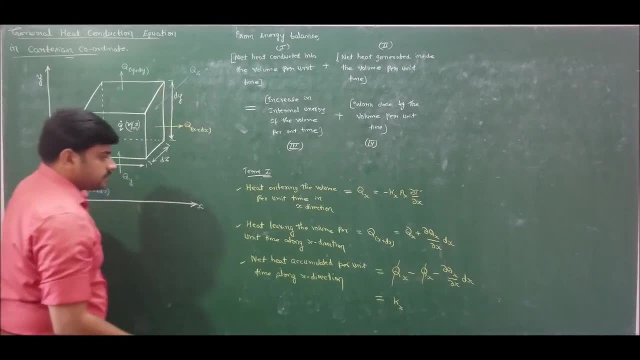 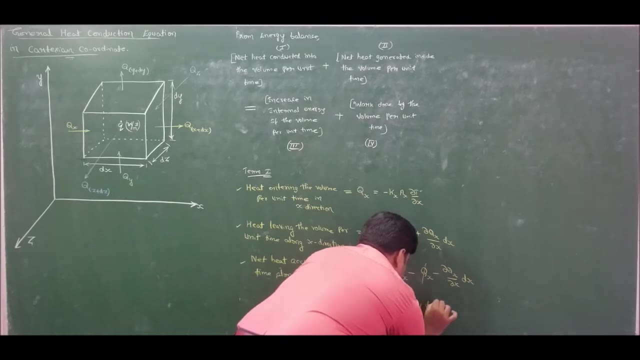 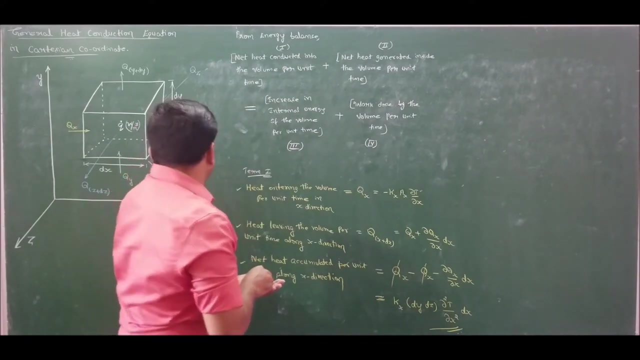 Area perpendicular to x direction will be dz, dy. So therefore area perpendicular is dy and dz Times. we have dou square t by dou x square dx, So this is the net heat accumulated per unit time along x direction. So, similarly, if I write: 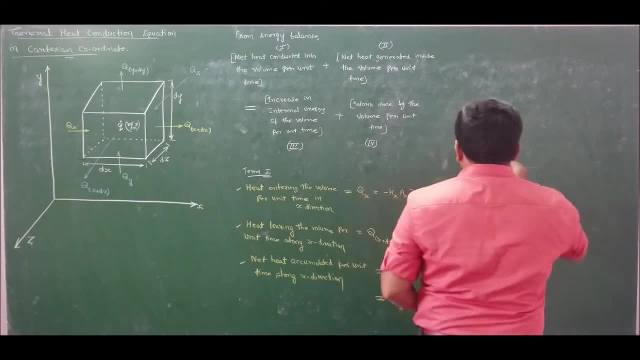 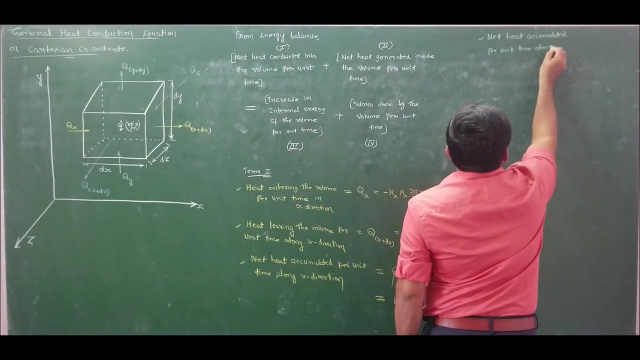 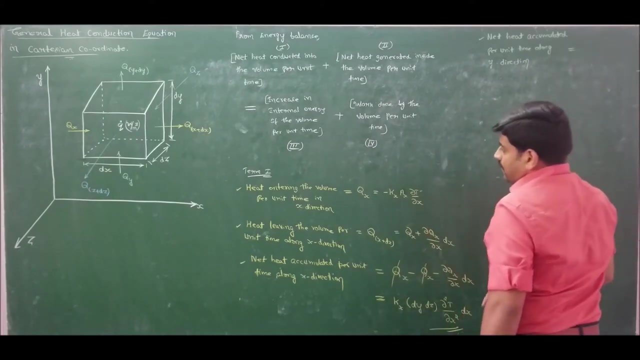 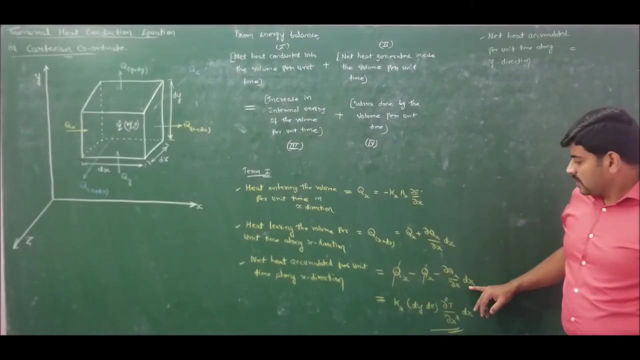 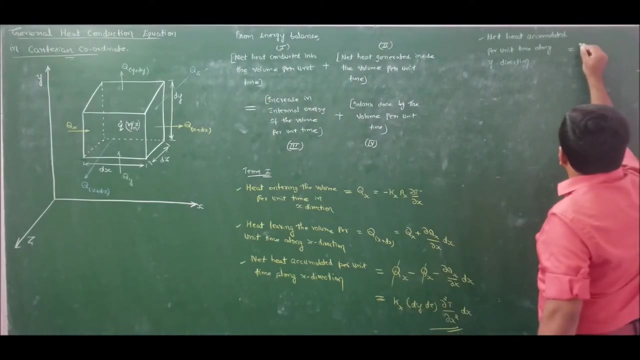 for y direction I get now. net heat accumulated per unit time along y direction will be equal to: it is qy minus qy minus dou qy. by dou y dy, I will cancel off qy and qy y, So remaining is this one. So therefore minus of minus is plus, So you get thermal. 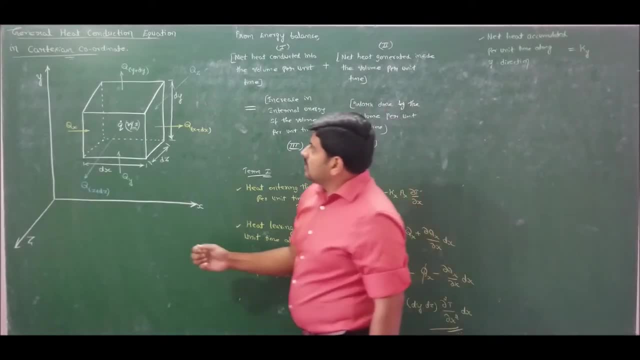 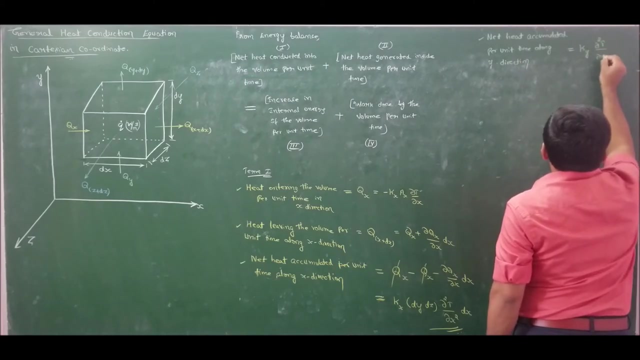 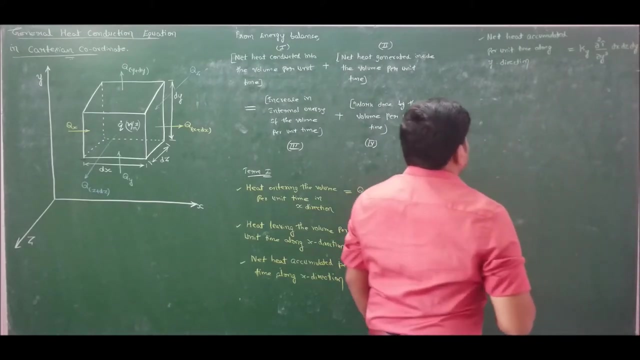 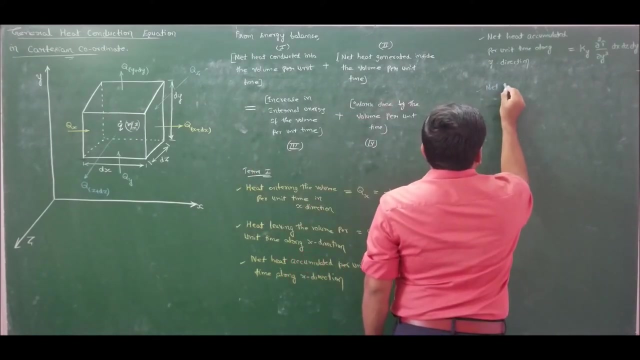 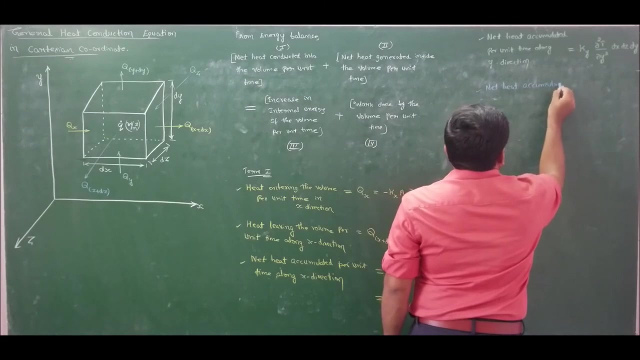 conductivity along y direction. Now, area perpendicular to y direction, Area perpendicular to y direction, will be dx dz. It is dx dz times. we have dou square t by dou y square: dx, dz, d y. Now, if I write the net heat accumulated per unit time along z direction will become: 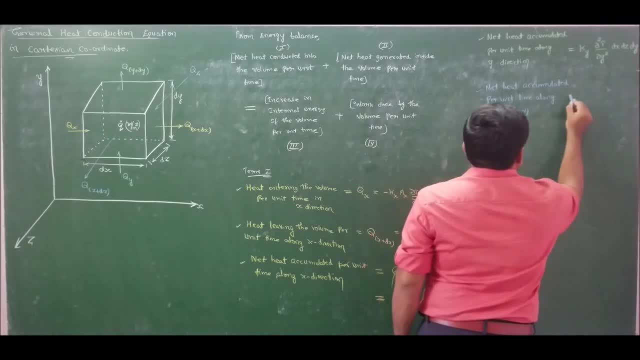 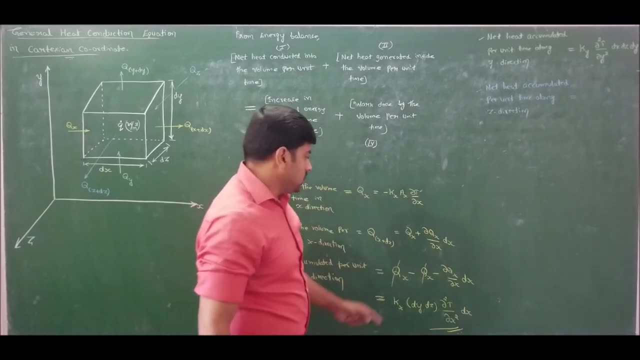 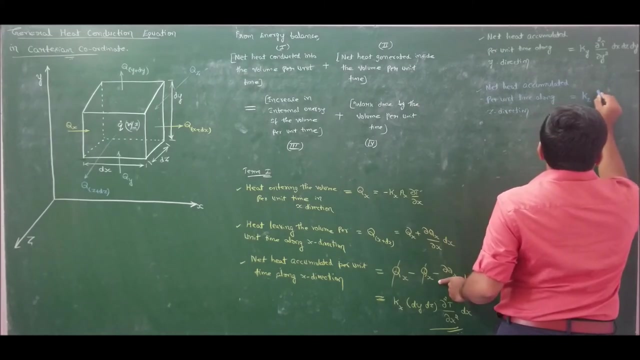 plus. So you can write this as qz minus, qz minus dou qz by dou z dz. So therefore qz qz will get cancelled, Minus of minus will become plus. It will become thermal conductivity along z direction dou square t by dou z square, Now, area perpendicular to the direction of. 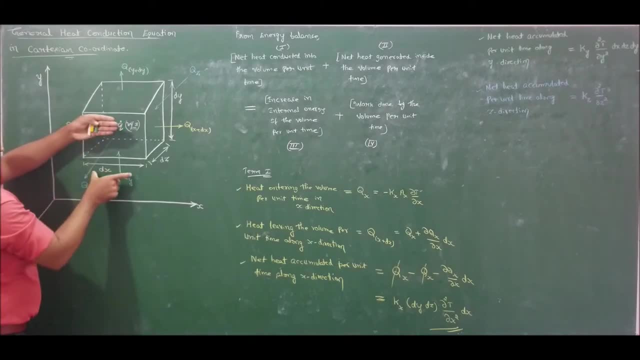 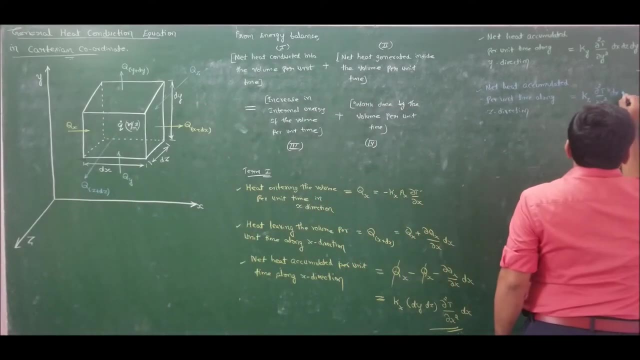 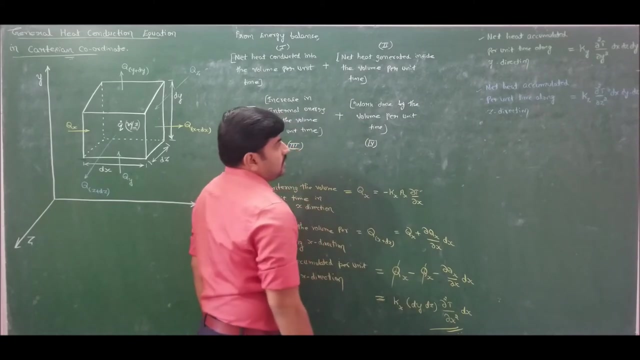 z Area perpendicular to the direction of z is dx, dx. So therefore area is dx, dy into dz, So dz is from this expression, Writing it along z direction. So therefore we have calculated what is the net heat accumulated per unit. 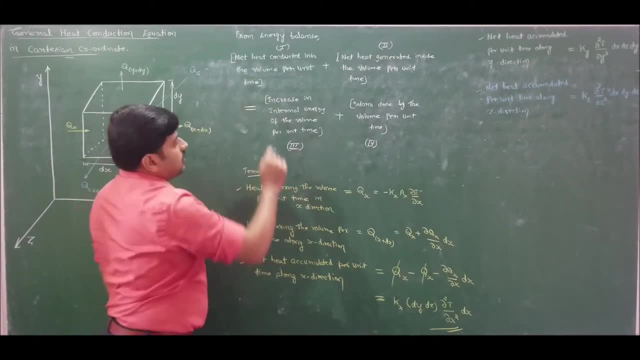 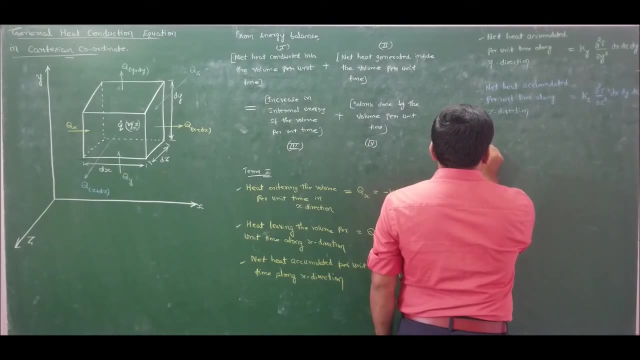 time along x direction, y direction and z direction. So therefore the total heat conducted from all the three directions will become So. therefore we have calculated the first term, that is, Let total heat conducted into the volume per unit time from all the three directions. 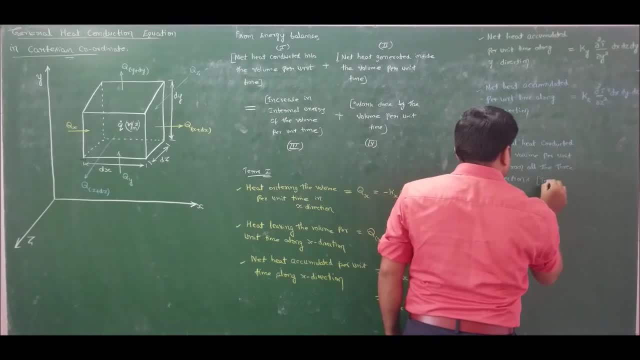 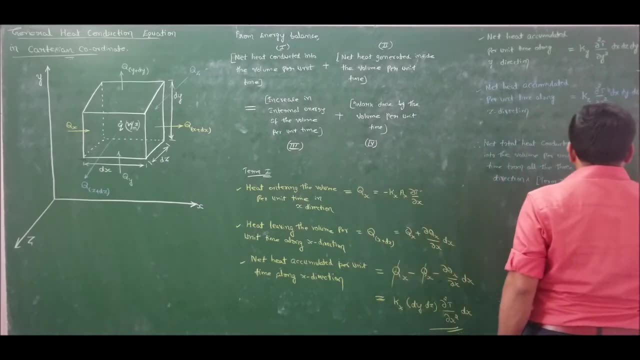 That is, Let total heat, Let total heat, Let total heat. The term 1 will be equal to along x direction. it is kx dou square t by dou x square. Let me take dx dy dz common plus ky dou square t by dou y square, plus kz dou square t by. 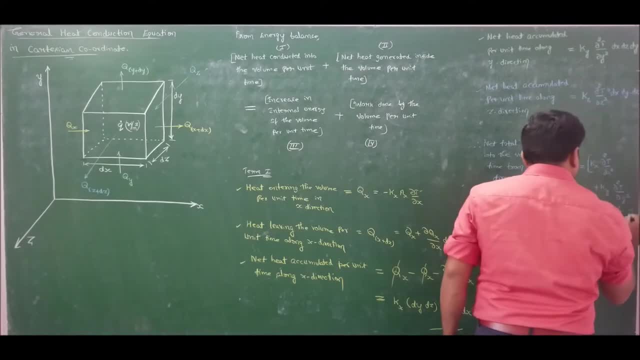 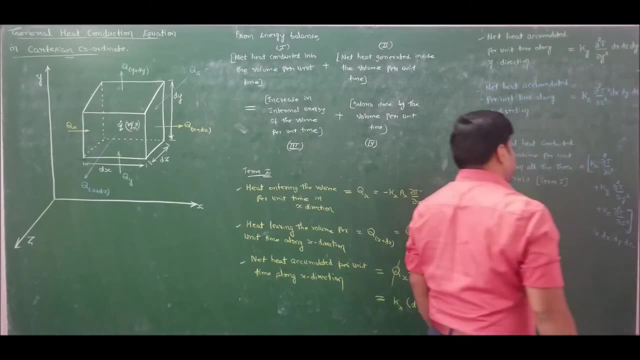 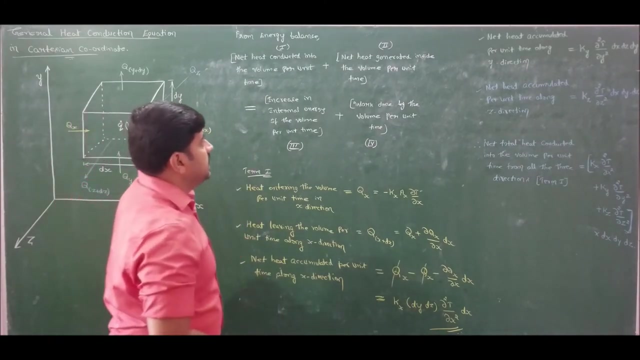 dou y square. Let me take dx dy dy dz, common plus ky dou square, t by dou y square, t by dou y square, t by dou z square, throughout I can take multiplied by dx dy dz. So this is what we have. Next coming for the second term: heat net heat generated inside the volume per unit. 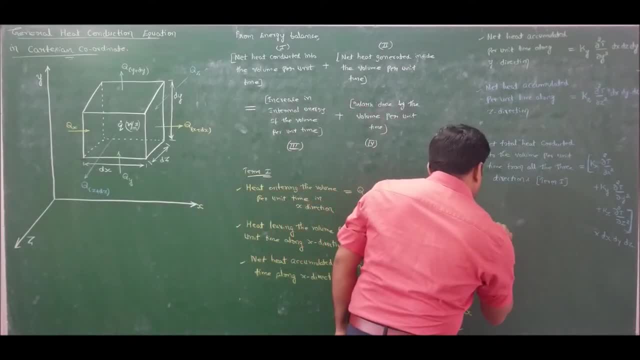 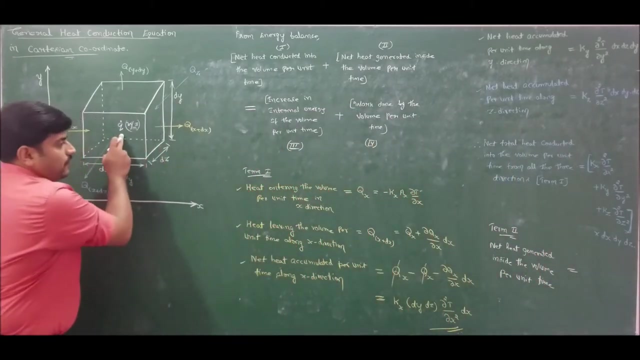 time. So if I go for term 2.. If I go for term 2, net heat generated inside the volume per unit time generated inside the volume per unit time will be equal to. we have Q dot wax per meter cube as heat generation, so I want it in wax, so therefore I should. 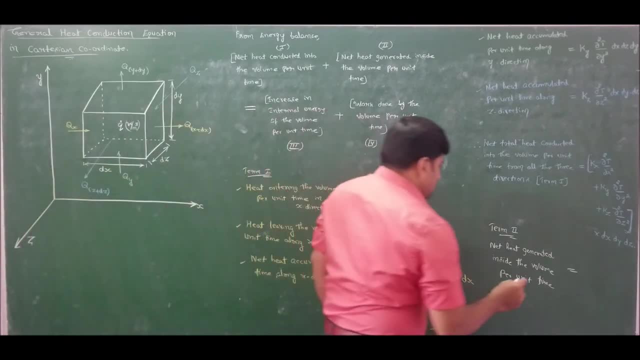 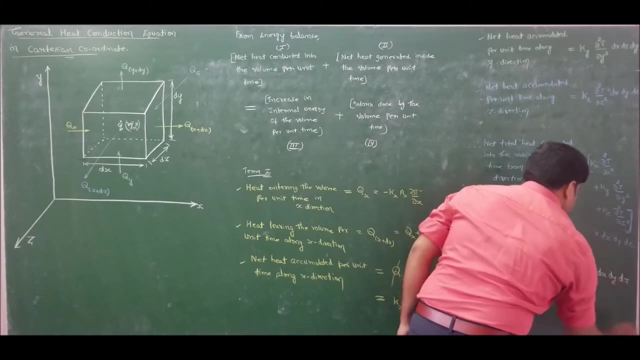 multiply volume meter cube. so therefore it is Q dot into volume is B, X, B, Y, B, Z, where Q dot is heat generated per unit volume, heat generated per unit volume per meter cube. so therefore it is Q dot into volume is B, X, B, Y, B, Z, where Q dot. 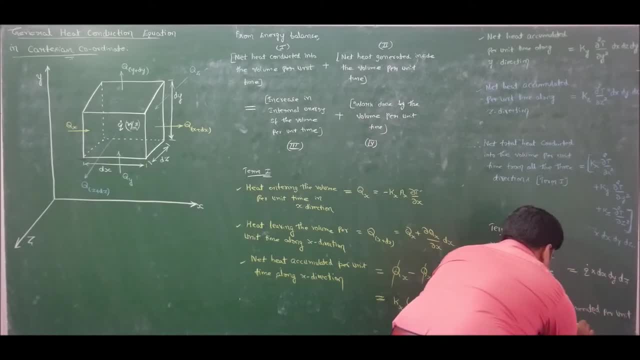 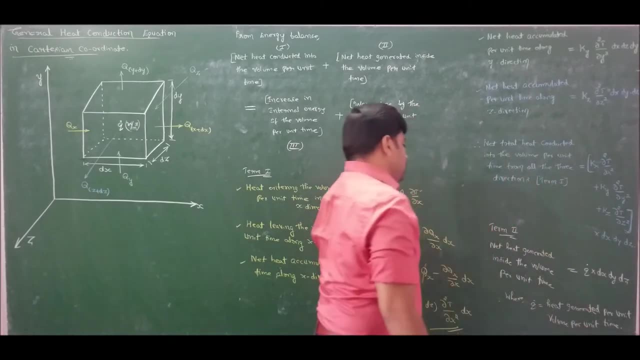 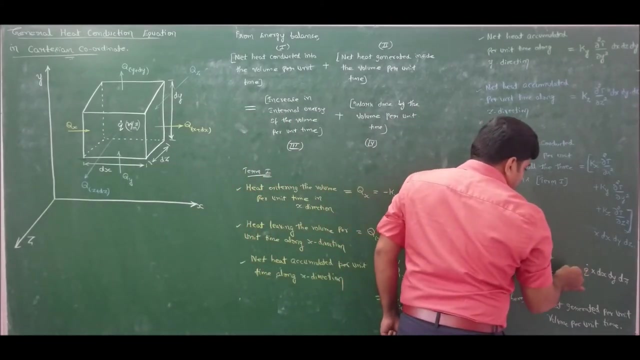 is heat generated per unit volume per unit time, which is in wax per meter cube. so I want net heat generated inside the volume per unit time. so therefore I multiply volume to the net heat generated per unit volume. so if I multiply volume I will get Q dot into B, X, B. 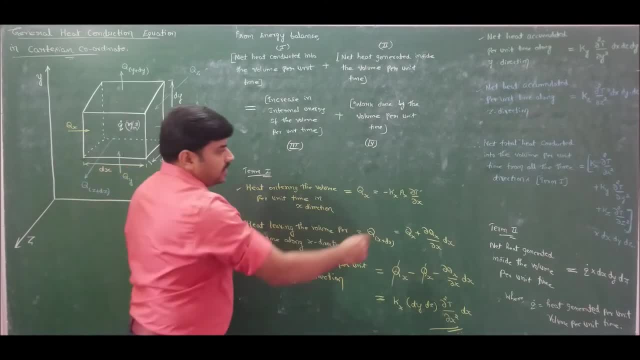 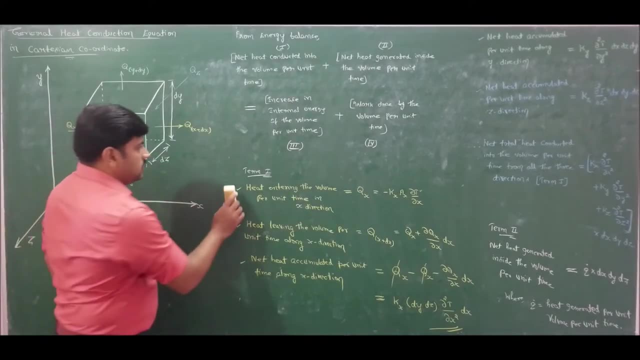 Y B Z. so we have done with term 1 and term 2. now moving ahead for term 3 and term 2. I have done with term 1 and term 2. I have done with term 1 and term 2. I have done with term. 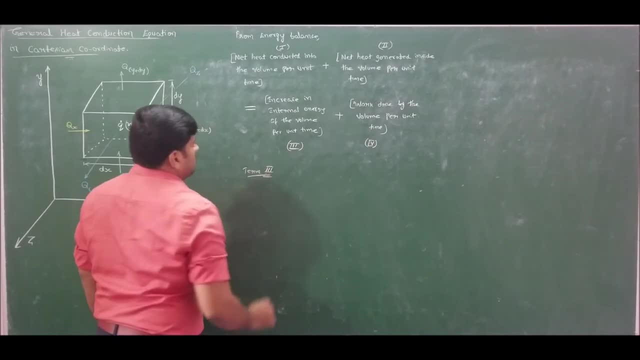 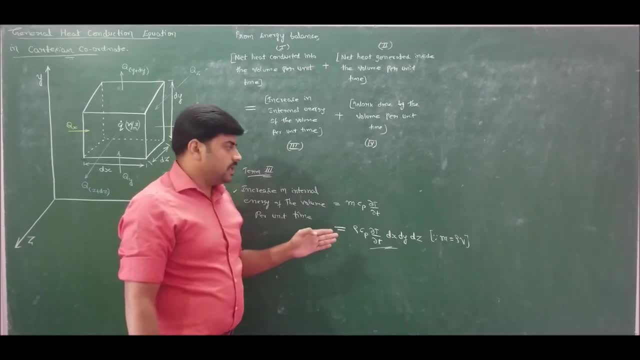 term 1 and term 2. I have done with term 1 and term 2. I have done with term 1 and term 2. I have is a function of space in more than one direction, and also it is a function of time. So now moving for the last term, that is, term 4, if I move for term 4, that is work done. 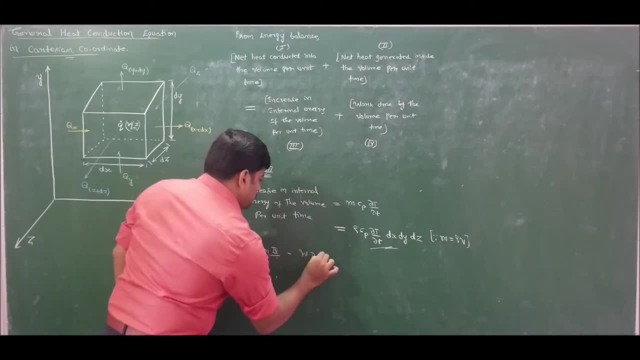 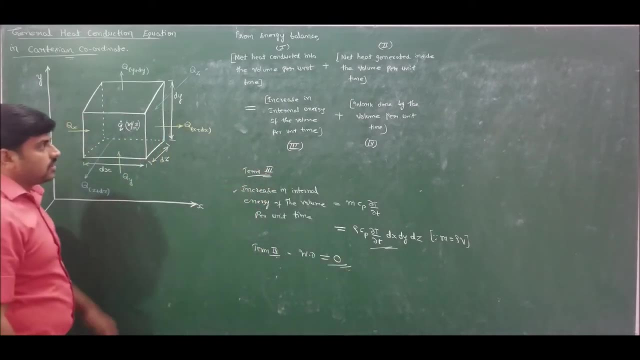 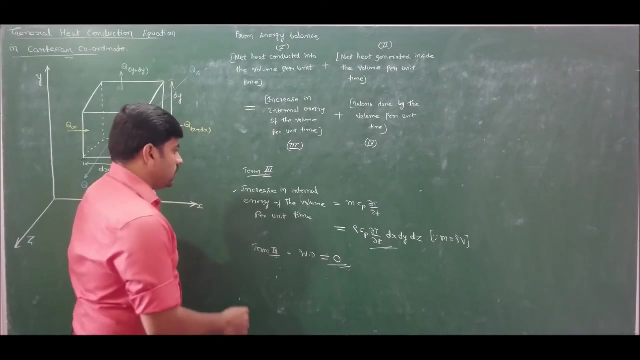 per unit time by the volume is equal to 0, because it is not doing any work. the volume is not doing any work, So therefore term 4 is equal to 0.. Now we have calculated term 1,, term 2, term 3 and term 4.. So therefore, substituting in: 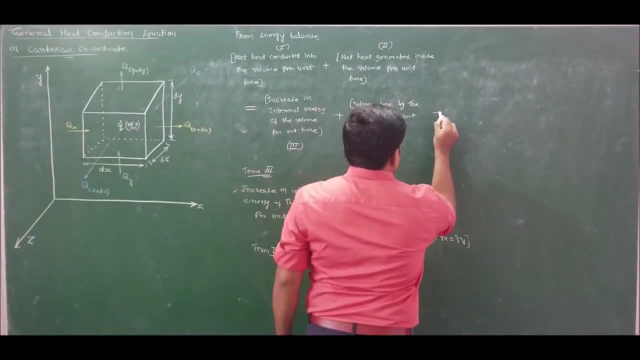 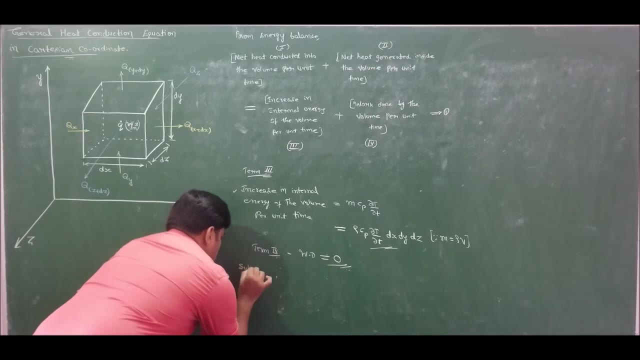 equation 1, let me take this as equation 1.. So substituting in equation 1, we will get. substituting in equation 1, we can write the net heat conducted into the volume per unit time. So this is written as kx dou square T by dou x square, plus ky dou square T by dou y. 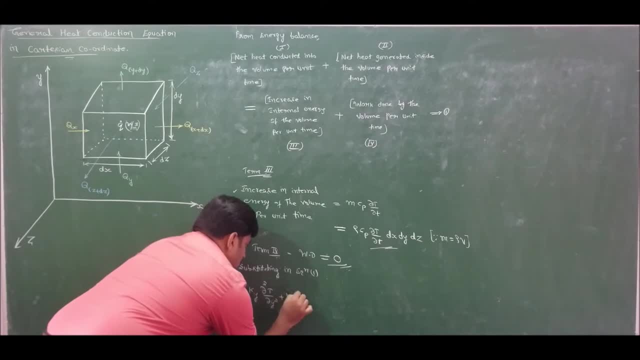 square plus kz dou square T by dou z square. So we have taken dx dy dz common. dx dy dz is the first term. Coming for second term, we know that it is q dot times: dx dy dz. This must be equal to increase in internal energy which is given by rho cp. dou t by dou t. dx dy dz plus term 4 is 0.. 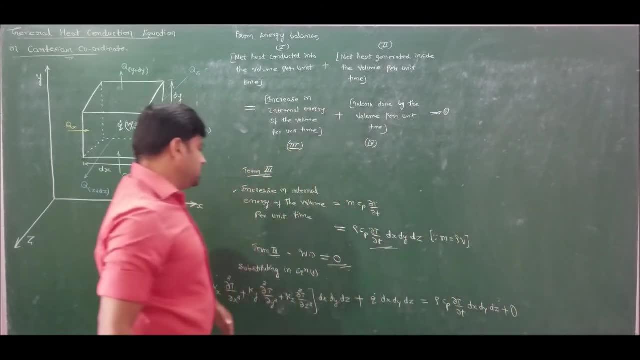 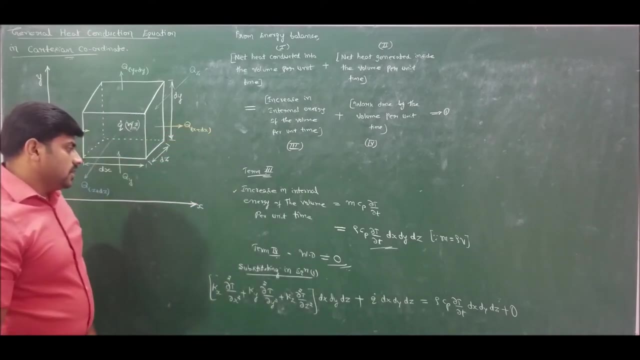 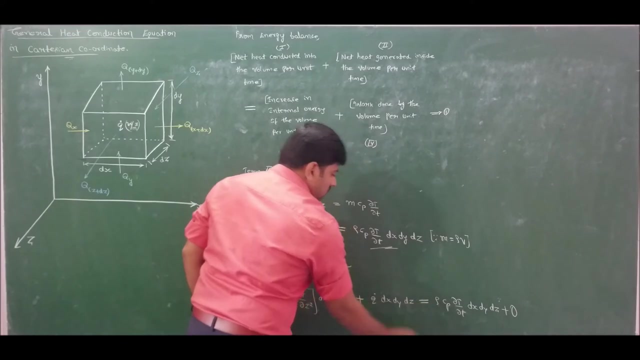 Okay, so this is what we got after calculating all the four terms individually and substituting to energy balance equation. So now I can cancel off dx dy dz by taking throughout comma. So I will take dx dy dz throughout comma and cancel off both in LHS and RHS. 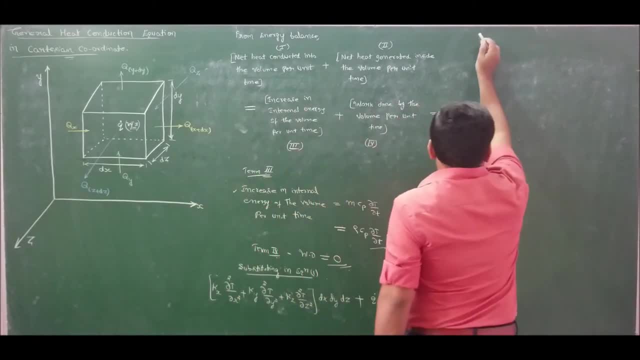 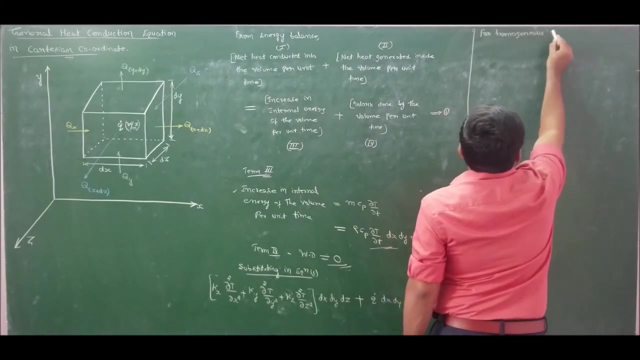 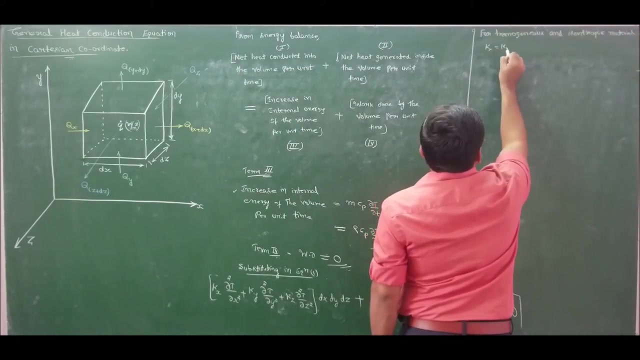 And if I consider the homogeneous isotropic material, so I will get the final expression. as for homogeneous and isentropic materials, We know that kx is equal to ky, which is equal to kz. are all same, I can call it as k. 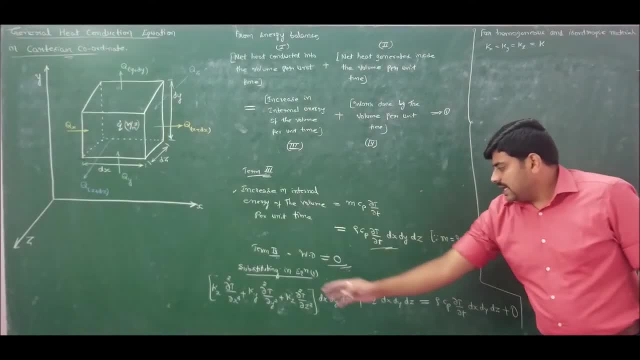 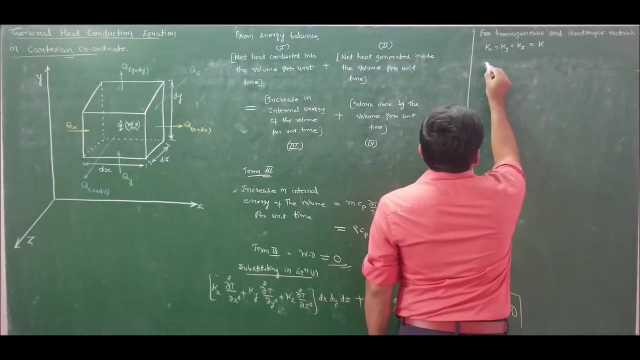 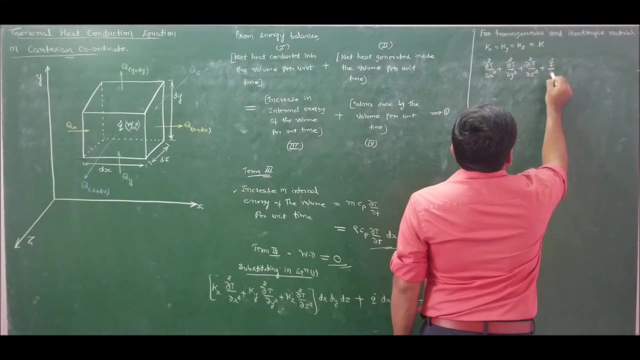 So what I will do is that I will take dx, dy, dz Throughout comma and cancel it off, and also I will take k comma and throughout divide this equation by k. So if I throughout divide this equation by k by taking k comma I left out, with dou square t by dou x square plus dou square t by dou y square plus dou square t by dou z square plus q dot by k is equal to: 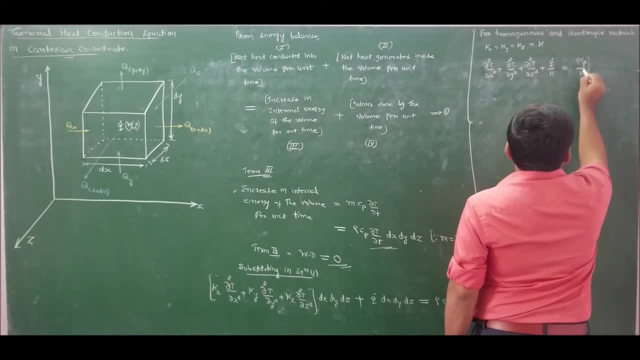 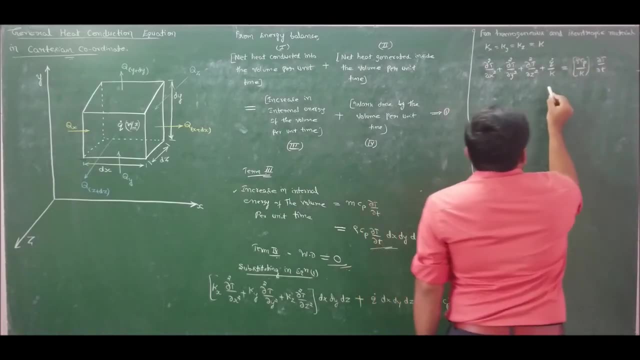 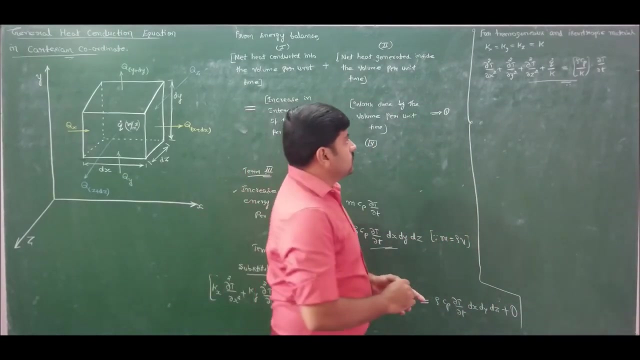 Hold on. I will play for the third time, So if I start from the denominator, I will continue from the denominator. I will repeat the previous previous expression for the second time. So what we have learnt is that in a three dimensional form y star, I will also find digital. 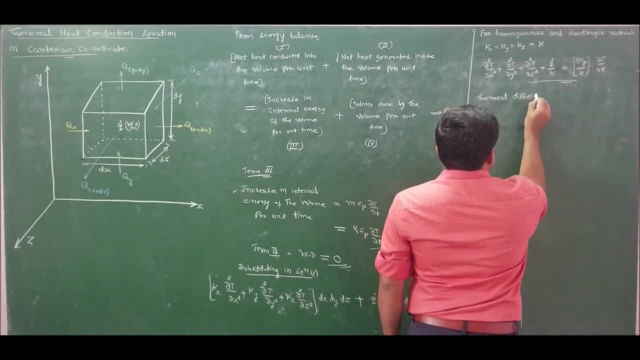 and then what we have learnt is that when unionuly- I am moving thing the unionarily of, we will find the union Far stop x, n and n square t minus 2 x square t. We will see that since we have taken all the terms asx, ends and meus, we will not find out. in general, 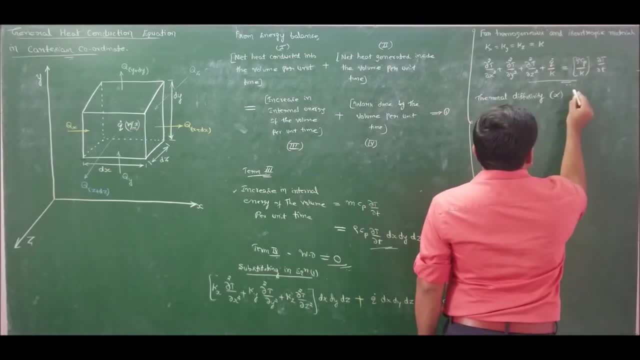 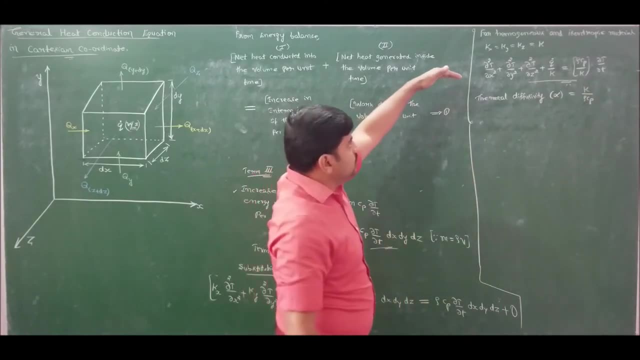 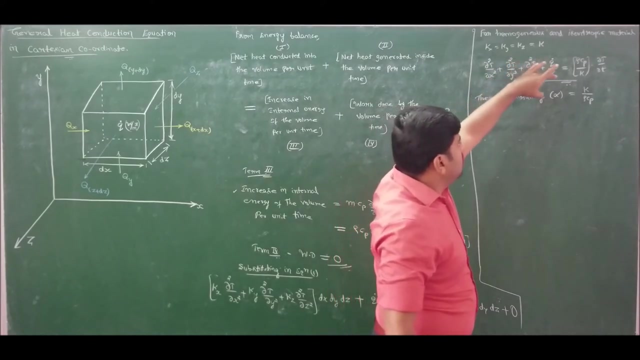 contradiction. So the term thermal diffusivity is alpha, which is equal to k by rho cp. So therefore this expression can also be written as: dou square t by dou x square plus dou square t by dou y square plus dou square t by dou z square plus q dot by k is equal to: 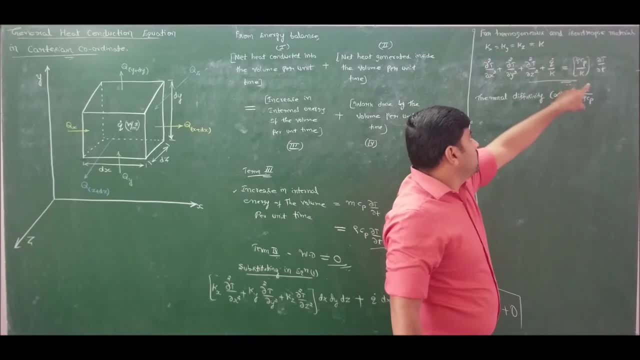 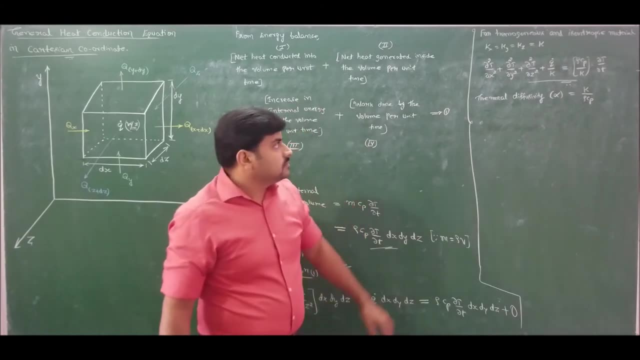 1 over alpha dou t by dou t. Because k by rho cp is alpha, it will become 1 over alpha dou t by dou t, Where the significance of thermal diffusivity is that it gives us an idea how fast heat can penetrate into the system. 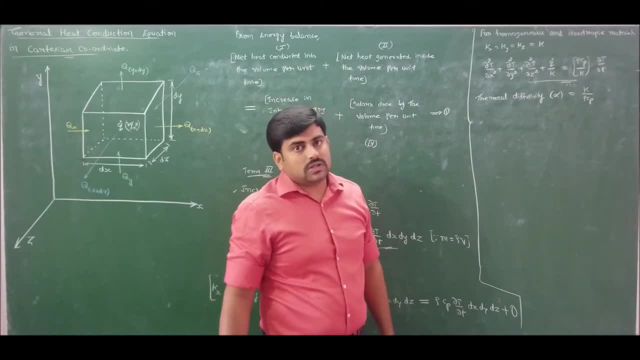 The analogous for thermal diffusivity is kinematic viscosity. So kinematic viscosity gives us an idea how fast viscosity is penetrated in the fluid. So, similarly, thermal diffusivity gives us an idea that how fast heat can penetrate through the system. 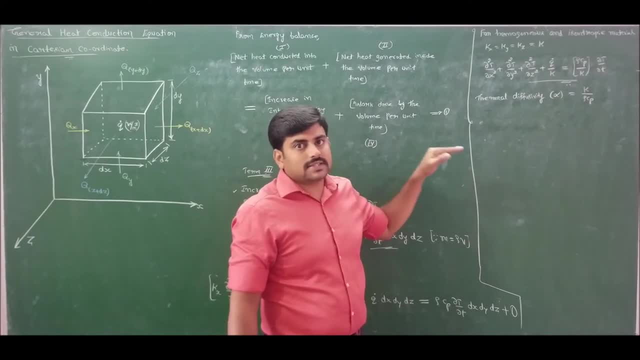 If thermal diffusivity is higher, heat flow in the system is faster. If thermal diffusivity is lower, heat flow in the system is slower. If thermal diffusivity is lower, heat flow in the system is faster. If thermal diffusivity is lower, heat flow in the system is slower. 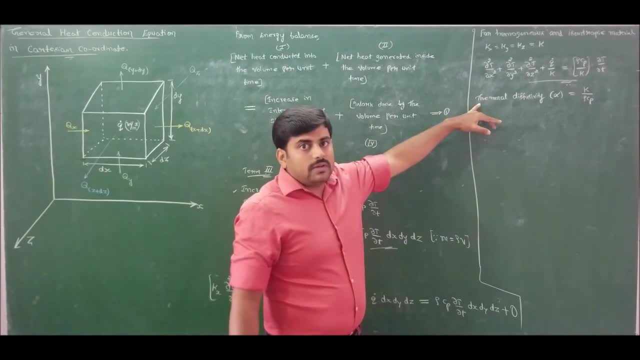 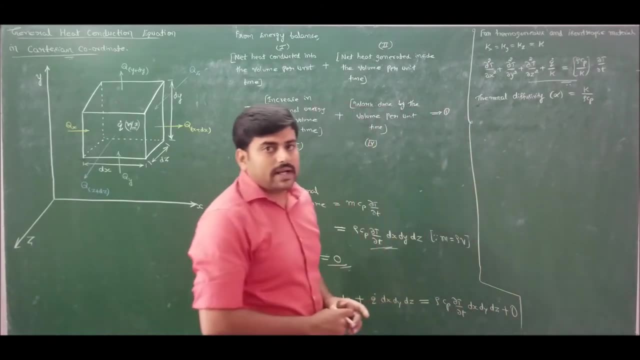 So therefore, higher the value of thermal diffusivity, faster will be the penetration of heat. So therefore, by knowing thermal diffusivity, we can determine how fast heat can penetrate in the given system. Now coming for special cases. 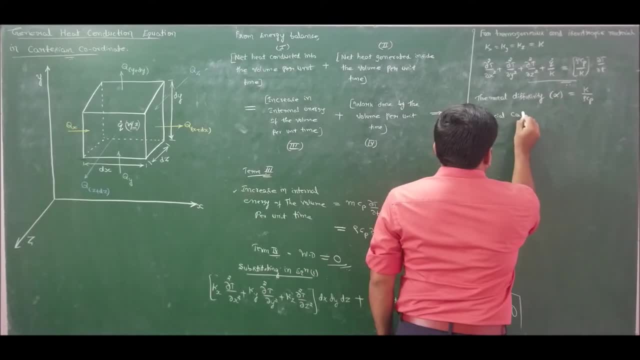 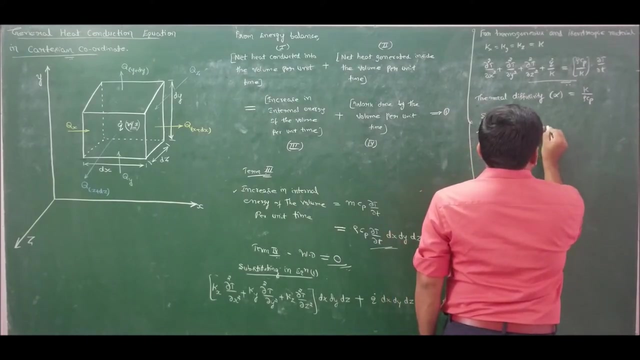 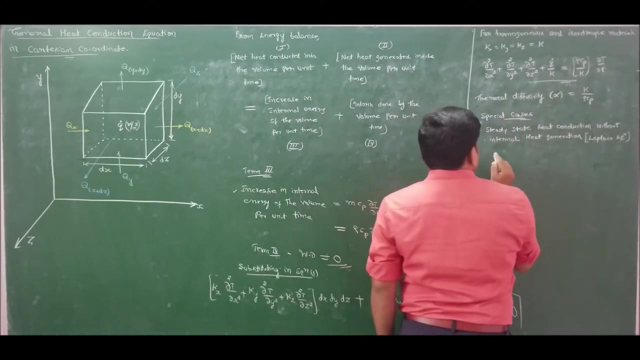 if I come for special cases. if I come for special case, first case is steady state heat conduction without internal heat generation, without internal heat generation. this is known as Laplace equation. this is known as Laplace equation, so Laplace equation is given. 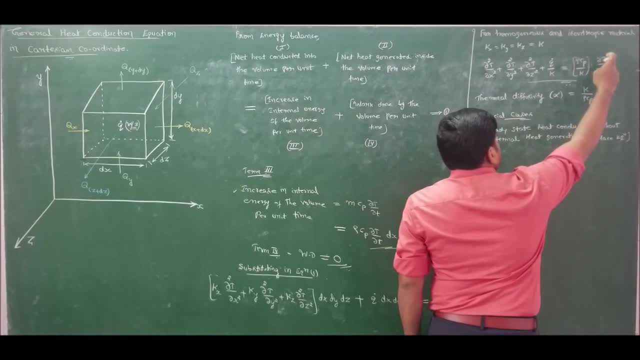 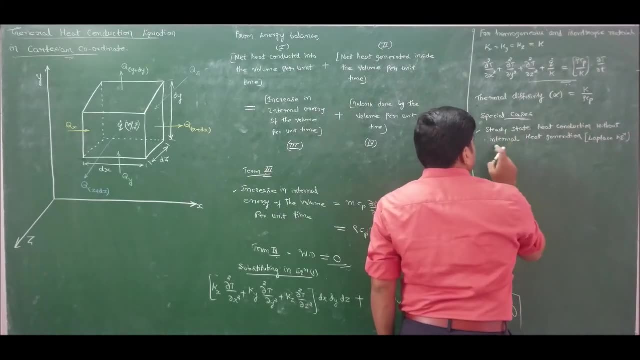 by for steady state. temperature is function of space alone. it is independent of time, so therefore derivative with respect to time will become zero for steady state and there is no heat generation inside the system, so therefore the second term will also become zero. hence the Laplace equation will become zero. 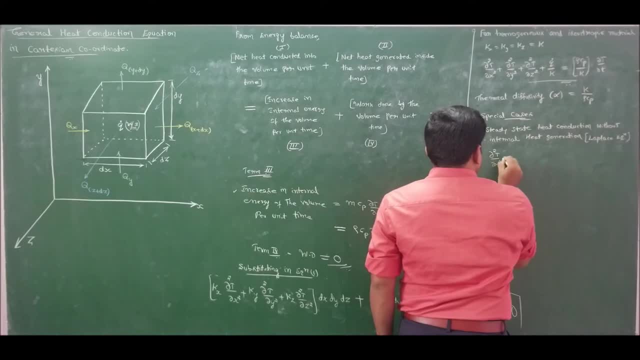 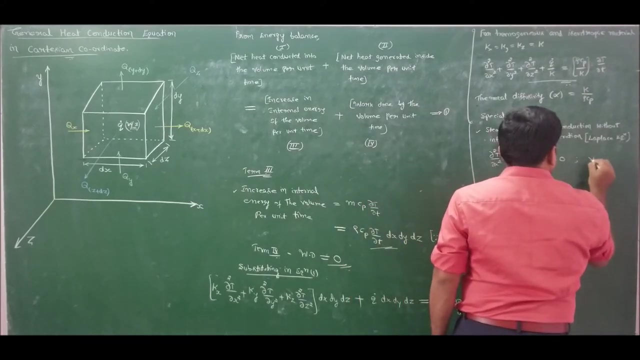 So the Laplace equation will become: dou square t by dou x square plus dou square t by dou y square plus dou square t by dou z square is equal to zero. so this is nothing, but del square t is equal to zero where del is called Laplace operator. 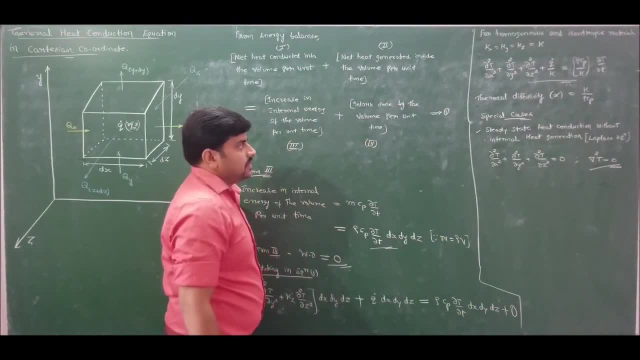 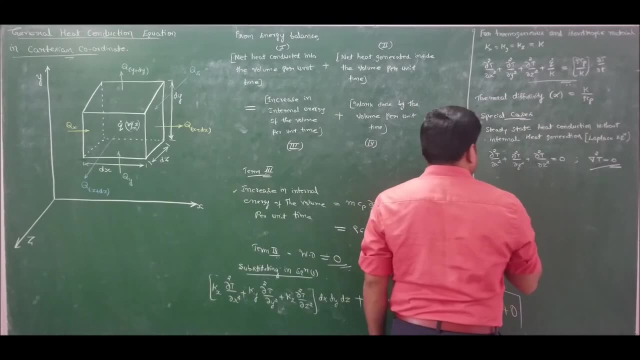 So this is about the special case, one that is Laplace equation, which is based on steady state heat conduction without internal heat generation. Now, coming for the second special case, that is, steady state with heat generation, we have steady state heat conduction with Á heat. 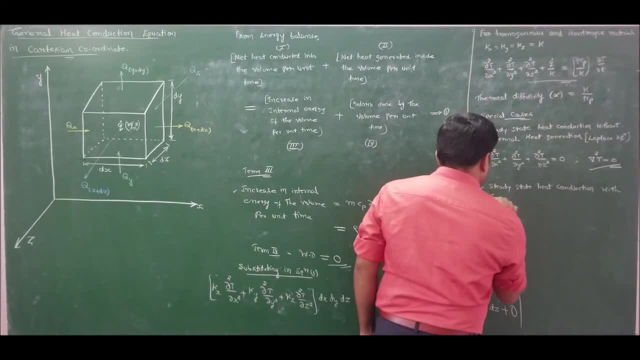 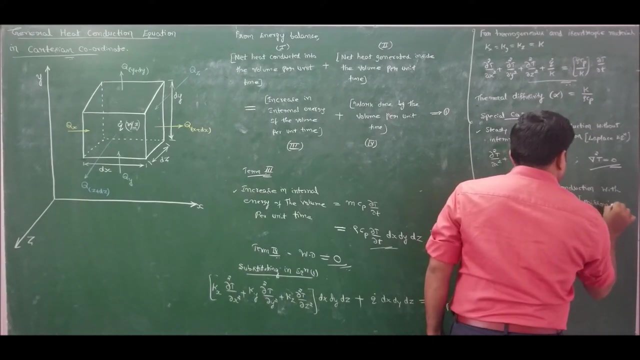 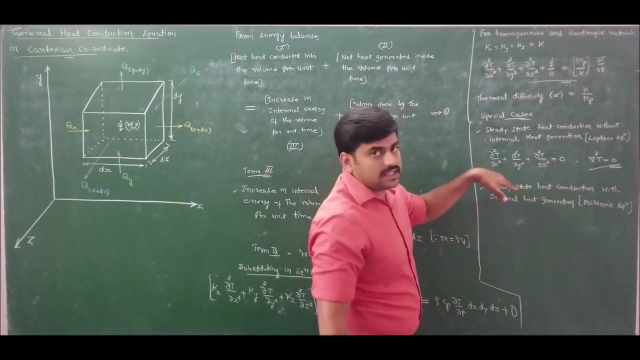 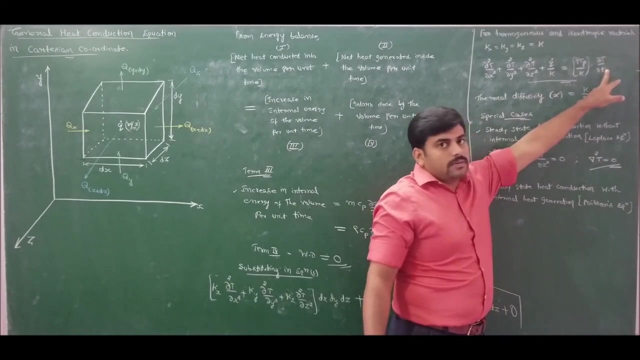 So This is known as Poisson's equation. coming for Poisson's equation, it is steady state heat conduction. Since it is steady state, temperature is function of space alone. it is independent of time. so therefore derivative of temperature with respect to time will become 0. 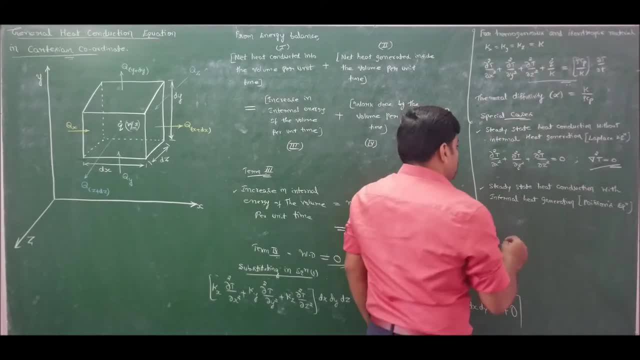 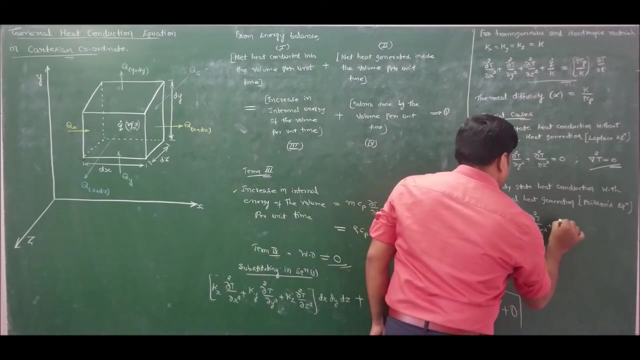 And we have internal heat generation. therefore the second term will exist. so Poisson's equation is given: by dou square T, by dou x square plus dou square T, by dou y square plus dou square T, by dou z square plus q, dot by k is equal to 0.. 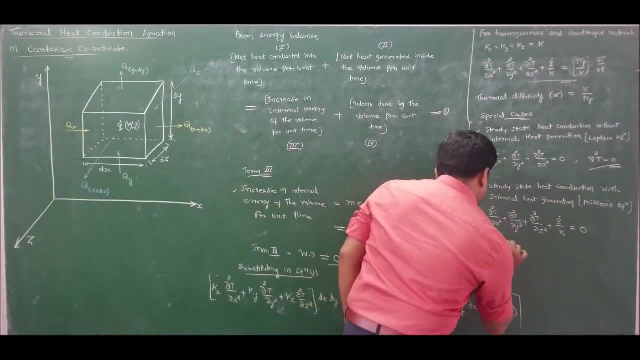 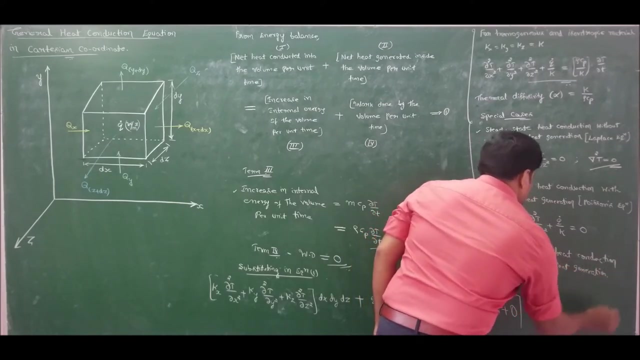 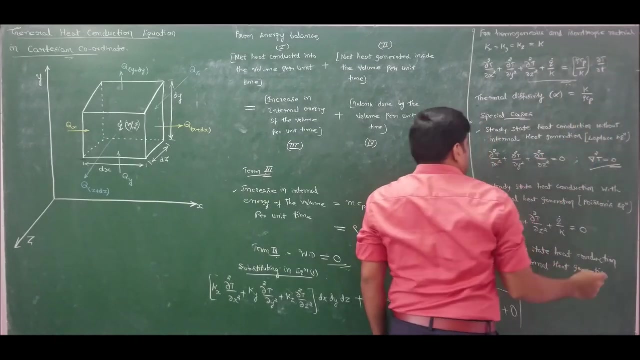 Now, finally, we have Unsteady state heat conduction. Unsteady state heat conduction without internal heat generation. without internal heat generation, which is steady state, termed as diffusion equation, Since it is unsteady state heat conduction: temperature changes with respect to time for transient, that is, for unsteady states, and there is no. 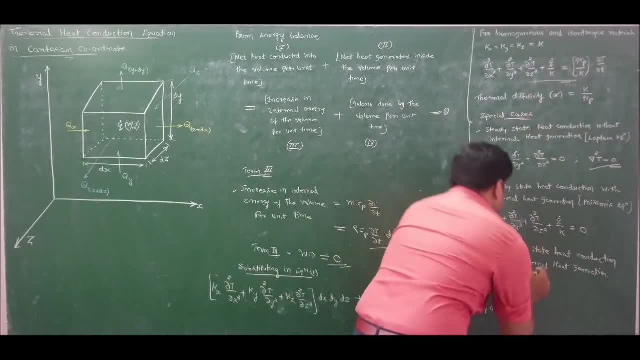 internal heat generation. Therefore, second term will become 0.. Hence the diffusion equation will be dou square T by dou x square, plus dou square T by dou y square, plus dou square T by dou z square, which is equal to 1 over alpha dou T by dou t. So this is known as 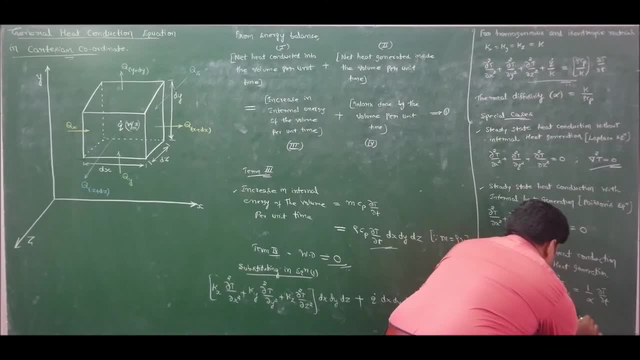 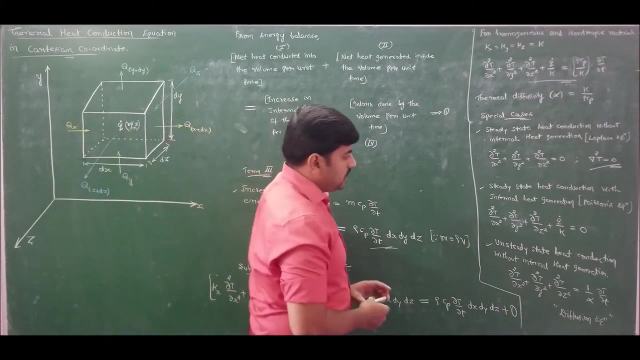 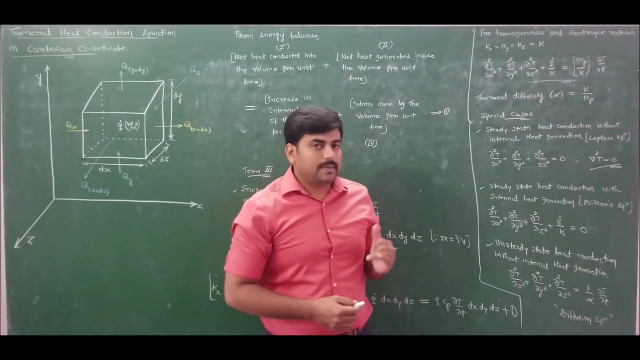 diffusion equation. So these are the three special case, that is, Laplace equation, Poisson's equation and diffusion equation for general heat conduction equation. Let me pause this video for a while so that people can copy it down. Later we will solve. 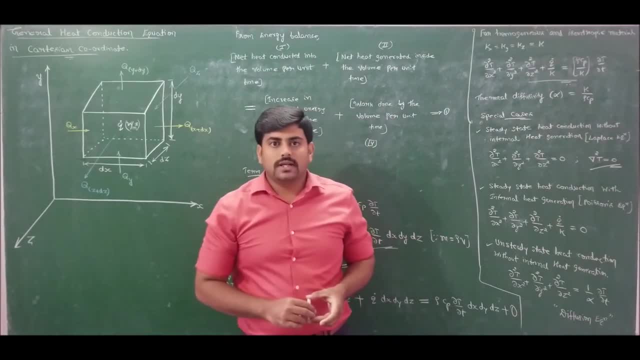 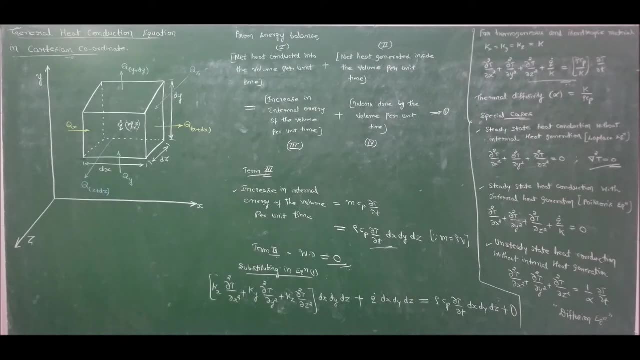 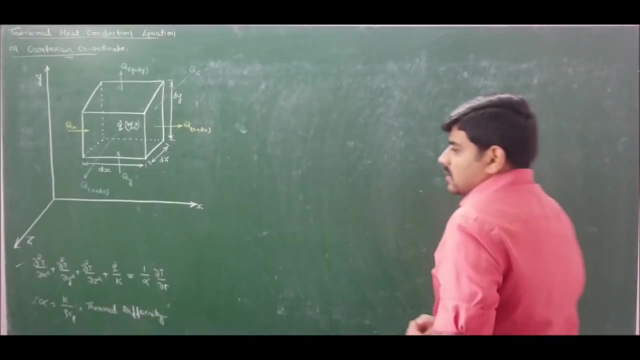 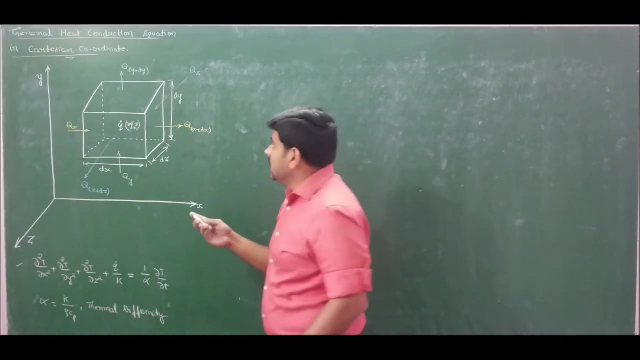 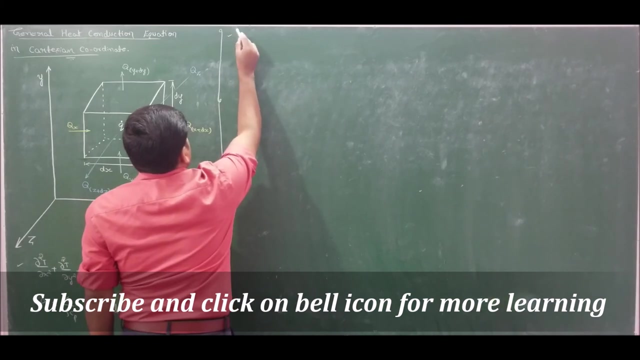 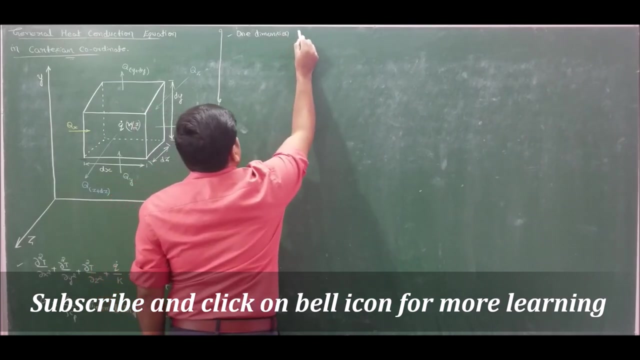 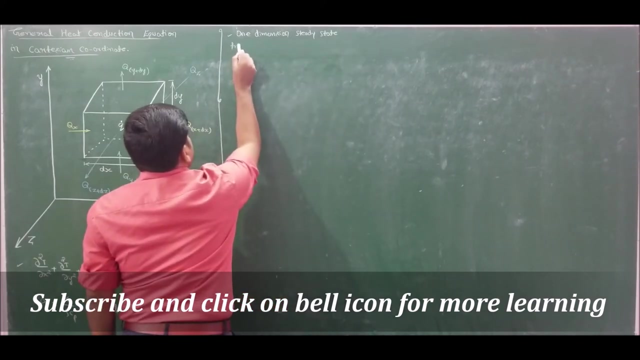 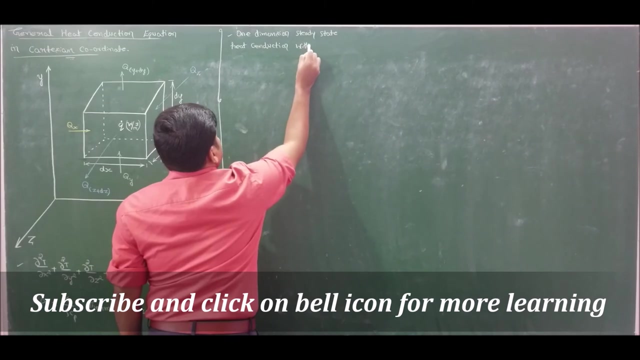 for one-dimension heat conduction in Cartesian coordinate for a plane wall. Now moving ahead for one-dimension steady state without internal heat generation: heat conduction equation analysis through a plane wall. we have the next topic, that is, one-dimension steady state heat conduction without internal heat generation. 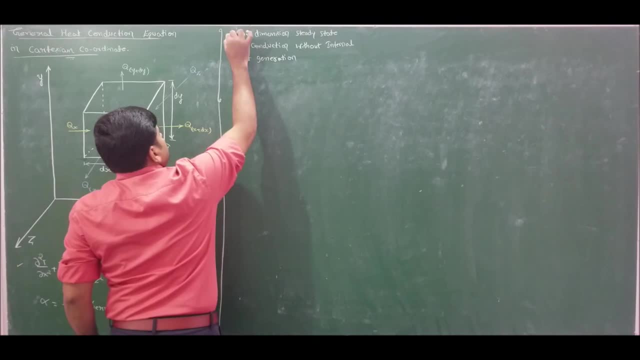 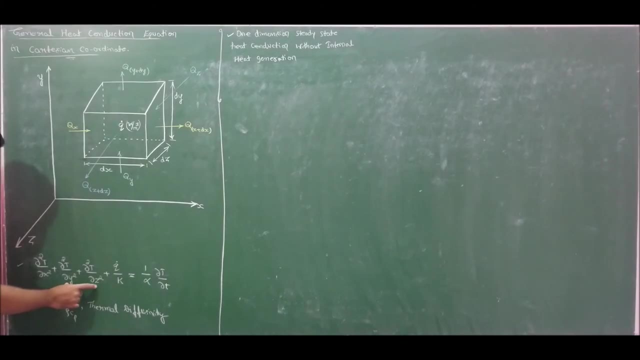 Now moving ahead for one-dimension steady state heat conduction without internal heat generation. as I said, it is one-dimension, So therefore y-direction and z-direction will be neglected. It is steady state, So therefore temperature is a function of space. 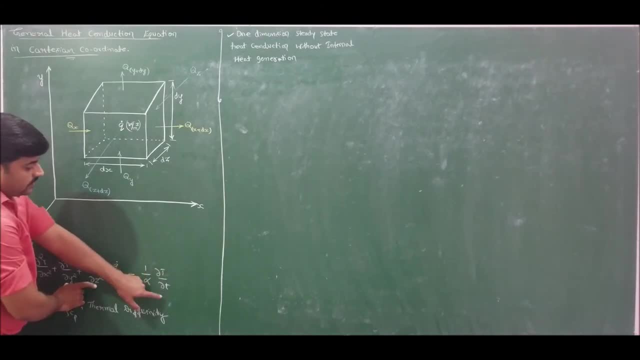 alone. It is independent of time. So therefore derivative of temperature with respect to time will be equal to 0. And we have no internal heat generation. Therefore the second term will also become 0. That is, q dot by k will also become 0. So therefore substantial. 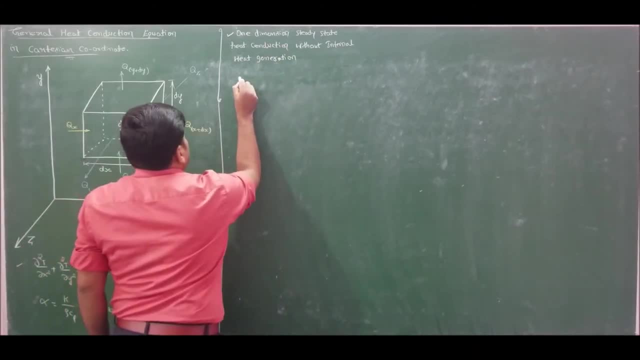 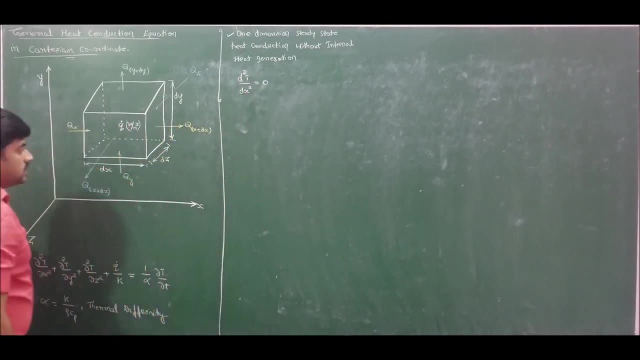 heat conduction value. Second term will be 0.. förstile one-dimension. let us define this equation. So, at this time, t falls to 0,. 0 does not apply, So t falls to x. So x is. 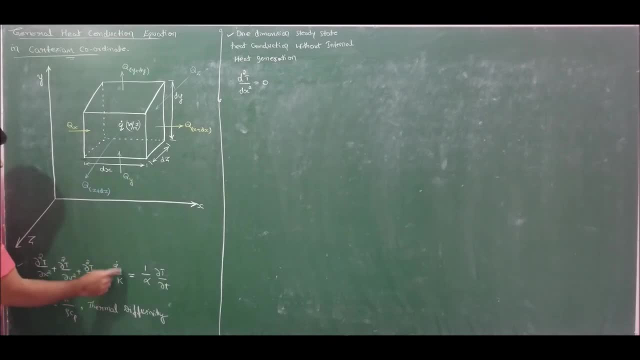 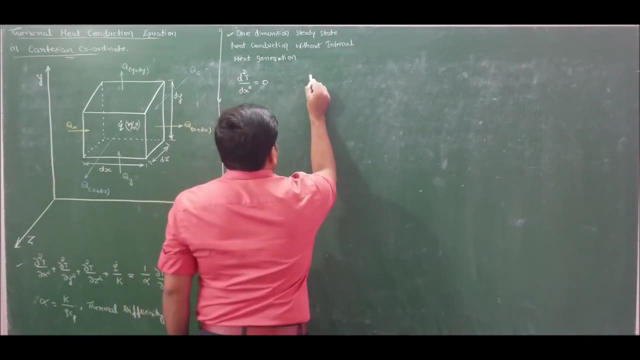 equal to 0.. Which�신e a given dimension If tیکin1,et z ヽ, So t Perdian 2.So I will get d2, t by dx2 is equal to 0.. So, since it is one dimension, 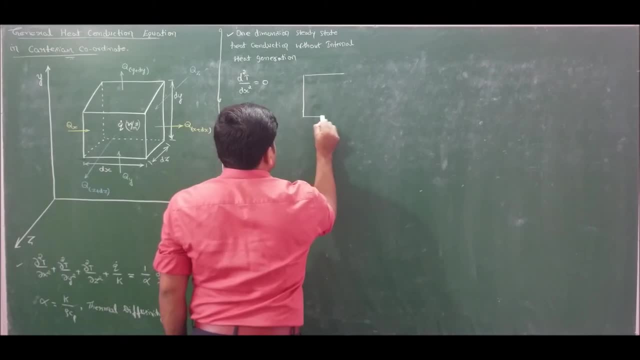 y and z direction are neglected. without internal heat generation, the second term will become 0, steady state, So therefore Rxs will also become 0.. Now this is for heat transfer through a plane wall. Consider a plane wall like this. We have a plane wall like this, Rxs the time. 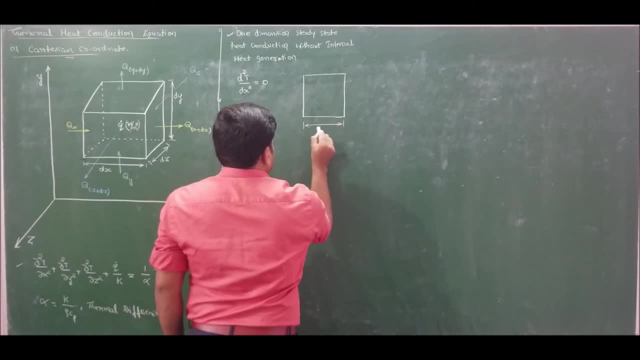 this: let the length of the wall be L and thermal conductivity be k. Now let the wall temperatures be T 1 and T 2, which are known to us, and we have a temperature gradient T 2 minus T 1 by L. Let us take this point as x is equal to 0, and this, as x is equal to 0. So this: 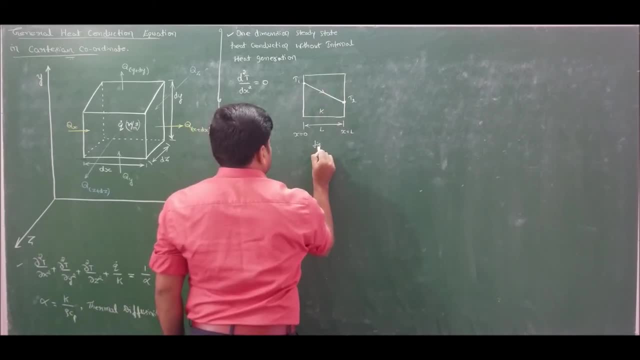 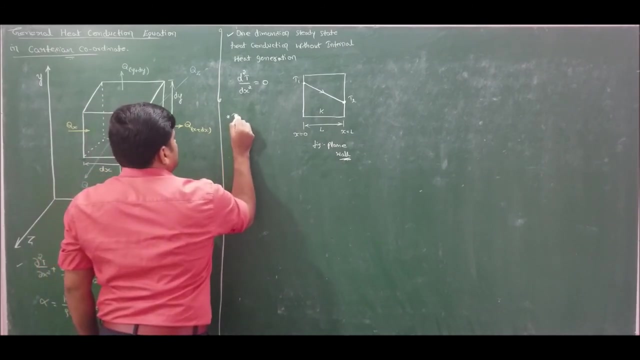 is L for a plain wall. Now I want the temperature distribution equation first. So therefore, we find temperature distribution. You have to find the general temperature distribution first. Let us take this as equation number 2.. Now to find the temperature distribution. 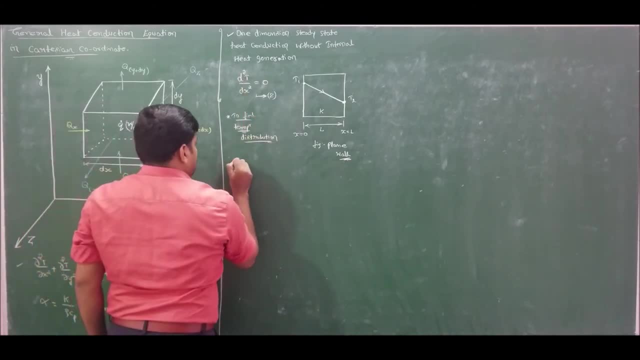 I want to integrate this equation twice, So, therefore integrating equation 2.. So if I integrate equation 2, I will get d. T by d. x is equal to 0.. So I have to integrate the constant of integration, C 1.. This is because of the reason: it is an indefinite integral. 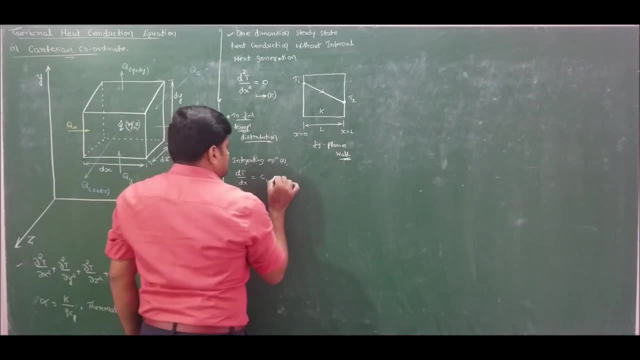 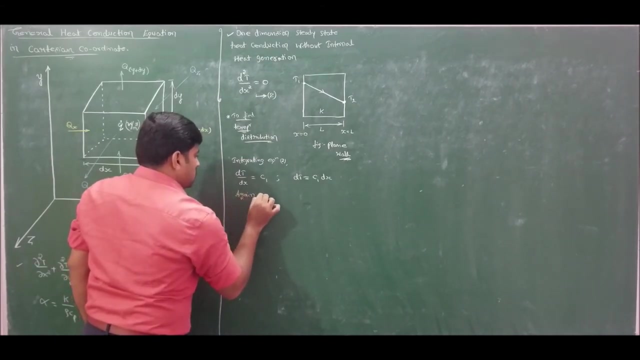 There is no limits for temperature. we have here. So let us take it as Now. let me rearrange this equation to the form d: T is equal to C, 1, d, x. Now again, if I perform integration, again, integrating the above equation. So if I integrate the above equation once again, 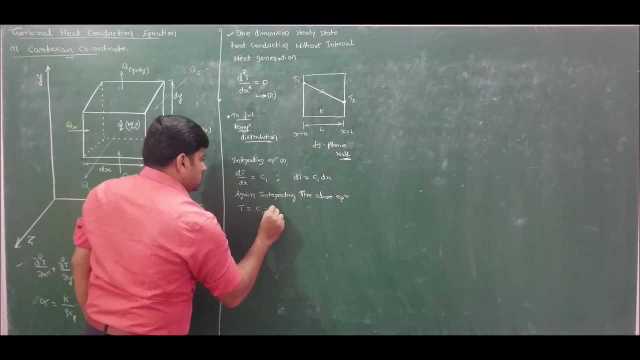 I will get temperature T 1 as C 1, x plus C 2.. Take it as equation number 3.. Now we have two constants: C 1 and C 2.. We have two boundary conditions at x is equal to 0 and x is equal. 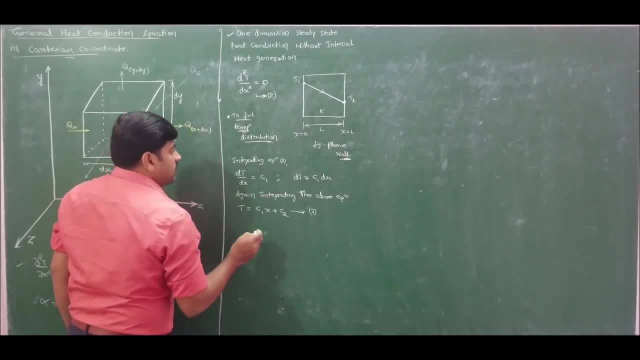 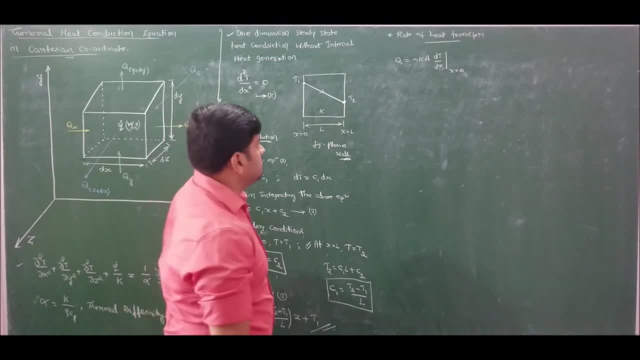 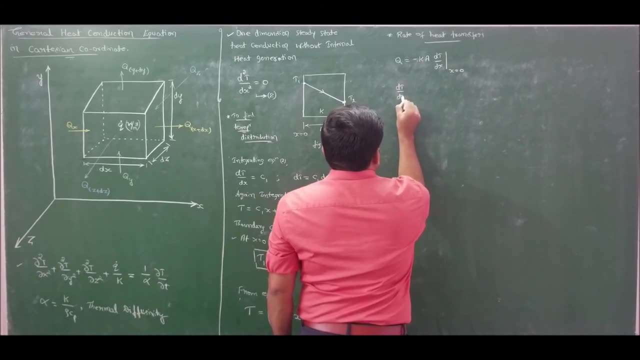 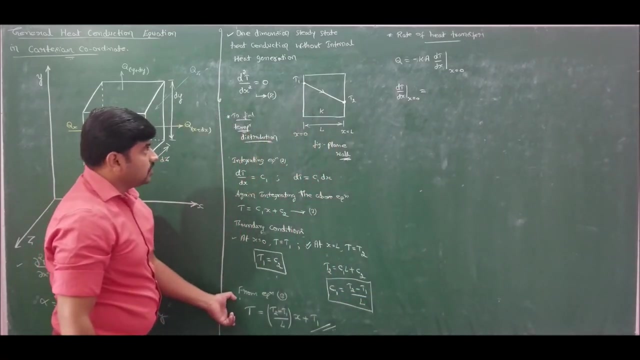 the temperature distribution and solve, you will get the answer. So if I substitute the temperature distribution and solve, I will get first. let me find dT by dx at x is equal to 0. So differentiating this by substituting x is equal to 0. we have differentiation of. 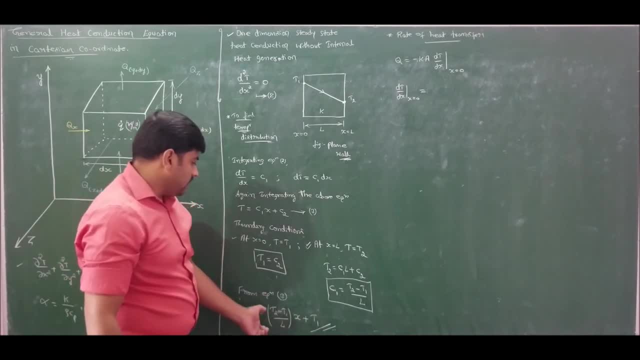 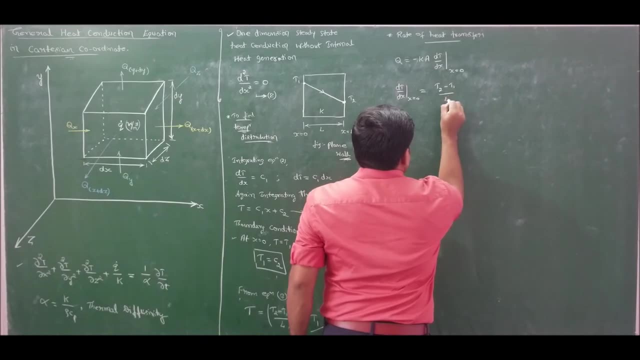 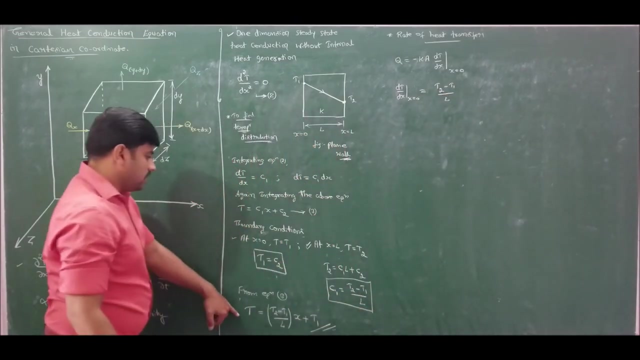 T1 is 0 because T1 is constant, independent of x. Now derivative of this is T2 minus T1 by L, that is T2 minus T1 by L. So this is the differentiation of temperature distribution, T, what we have. So now substitute this rate of free transfer equation, we will get Q is 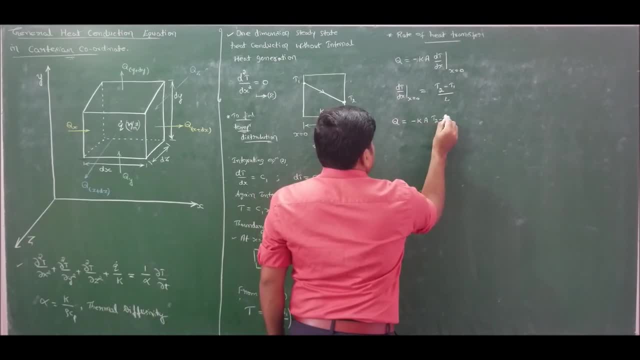 equal to minus Ka, T2 minus T1 by L. So multiply negative sign inside. So therefore rate of free transfer will become T2 minus T1 by L. So this is of the form: Q is equal to T1 minus T2 divided by L, by Ka, which we already discussed. 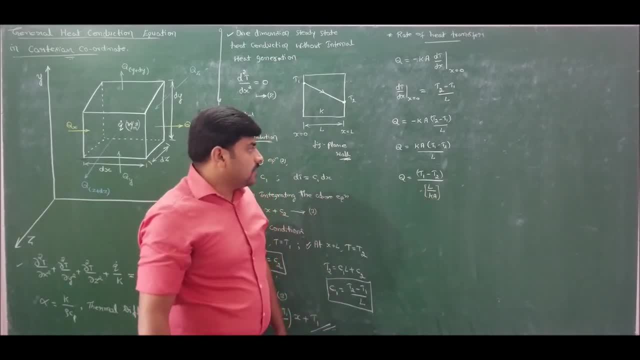 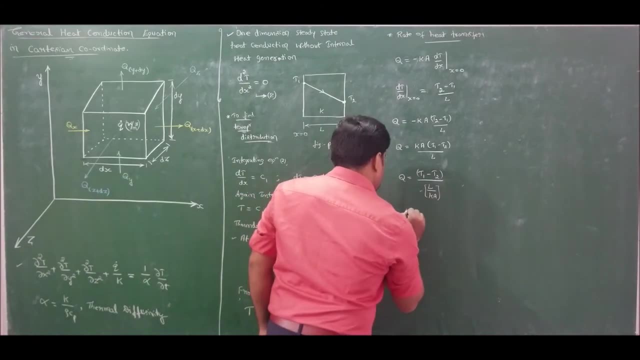 in our previous lecture. This L by Ka is thermal resistance for flow of heat due to conduction for a plane ball. So this is of the form. I is equal to delta V by electrical resistance, T1 minus T2 by L. So this is of the form. I is equal to delta V by electrical resistance. 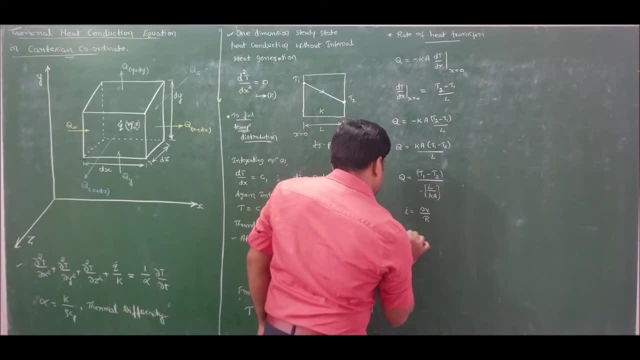 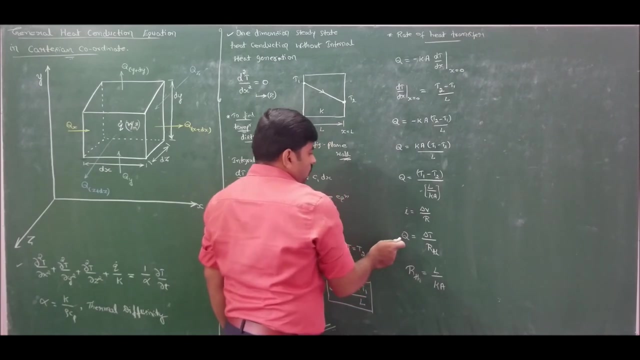 R. So therefore I can write: Q is equal to delta T by R thermal resistance due to conduction, where R thermal resistance for a plane ball is given by L by Ka. So flow of current is equal to difference in voltage by resistance- electrical resistance- whereas flow of heat. 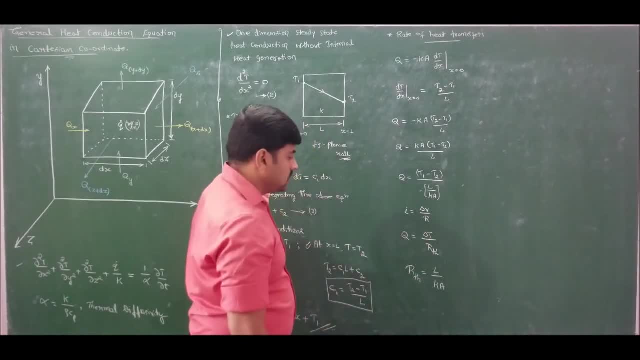 is equal to difference in temperature divided by thermal resistance. So comparing T2 minus T2 by R thermal resistance to T2 minus T2, by our contact force to heat transfer, ganzen heat transfer, we can state that thermal resistance is given by L, by Ka for conduction mode of 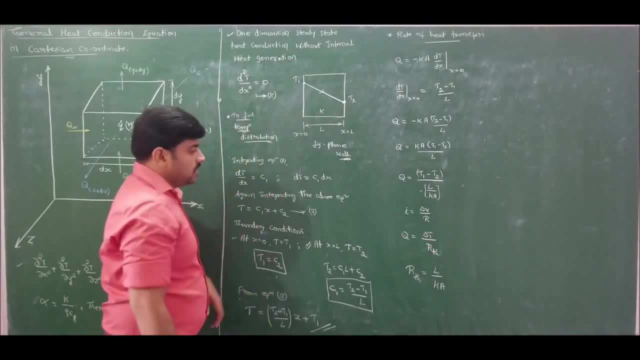 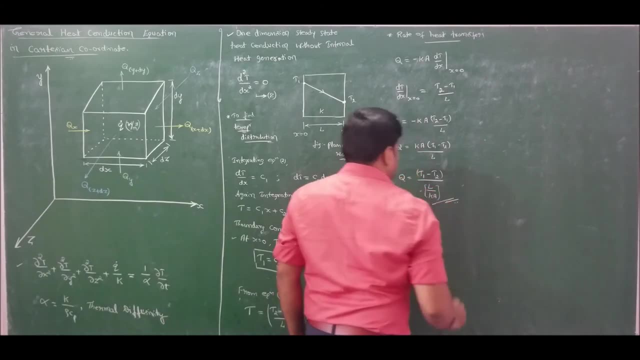 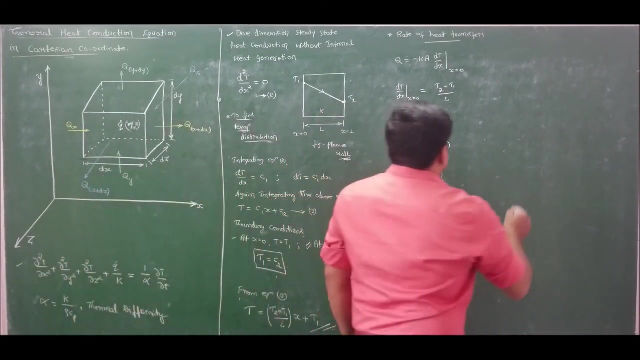 heat transfer through plane ball. So this is the expression for temperature distribution and rate of heat transfer, for heat transfer through plane ball in Cartesian coordinate system. Now if I move for composite wall, if I move for composite wall, I can write for composite wall as I am going to take thezet to. I am 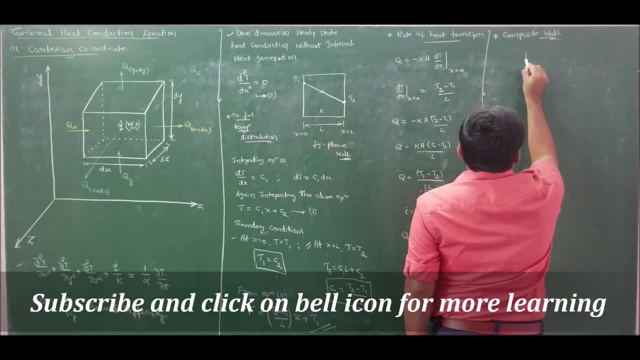 Let me consider a composite wall like this, having made of two different materials subjected for convective heat transfer on both sides. Let us take this point as 1, this point as 2, this point as 3, this point as 4 and this: 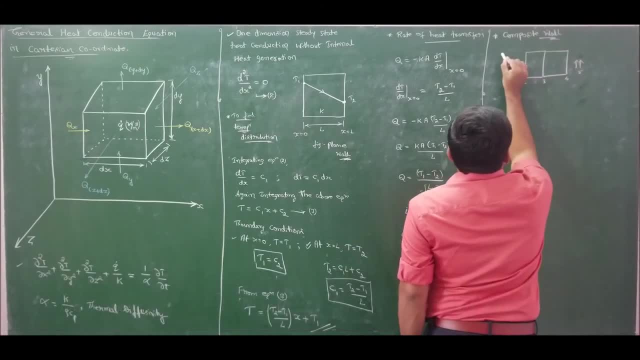 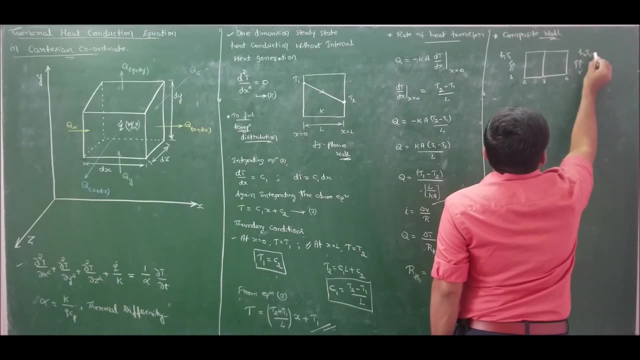 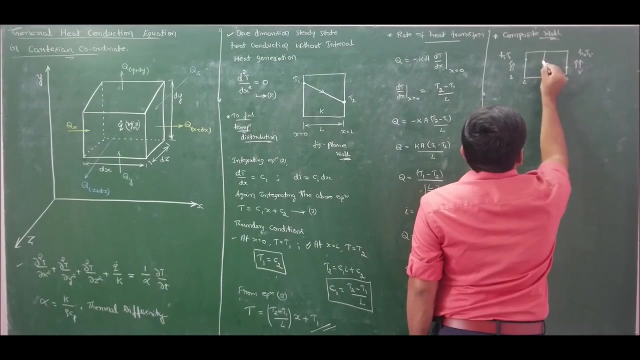 point as 5.. Let us call the convective heat transfer coefficient as h in R T1, this as h outer T5, and we have the variation of temperature from T2 to T4. Let me have T3 here. So like this, let us consider the temperature distribution. 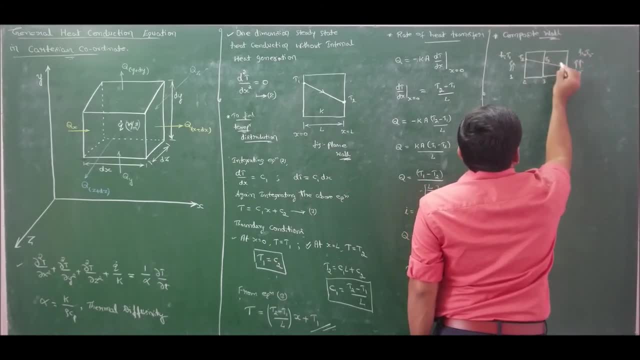 Here the temperature might be taken as T2, T3 and T4. like this: Let the thermal temperature be equal to T2.. Let the thermal conductivity as K1 and the area of first wall as A1.. For second wall, I will take thermal conductivity as K2 and area as A2, let the thickness of 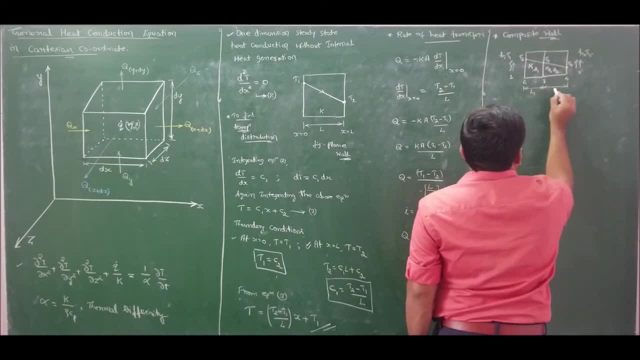 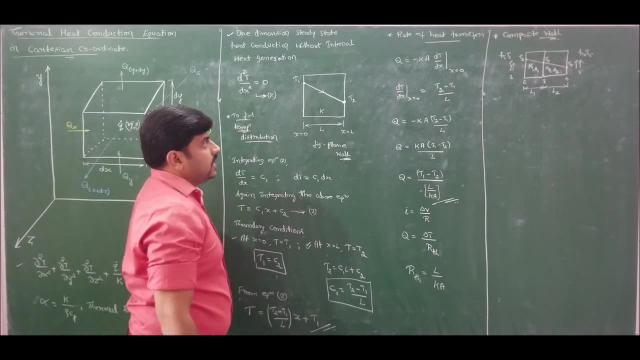 first wall be L1 and thickness of second wall be L2. like this, Let us consider a plain wall, plain composite walls, subjected for end deconvection on both sides. Let heat propagates from left end to right end. We will assume T1 is T2.. 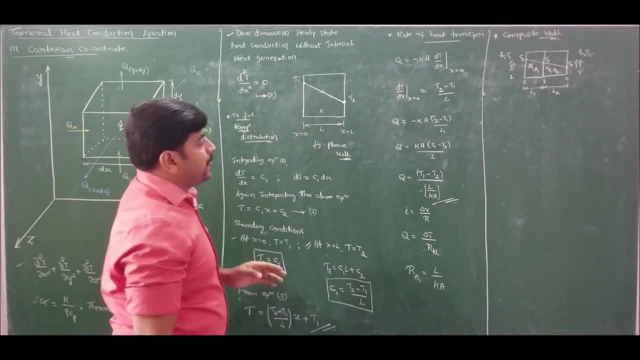 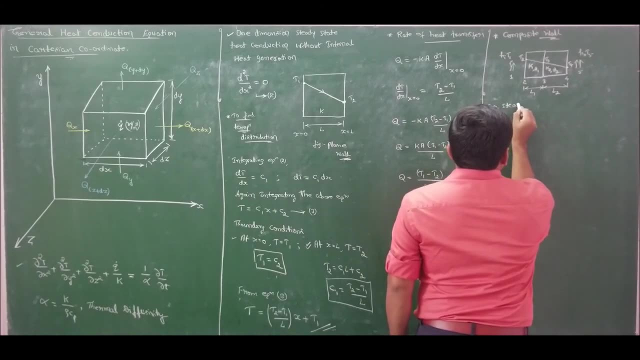 We will assume T2 is T2.. Let us consider the state of the end deconvection. Let us consider the state of the end deconvection on both sides. This is very, very high compared to T5.. Now for steady state. we know that for steady state, q is constant. 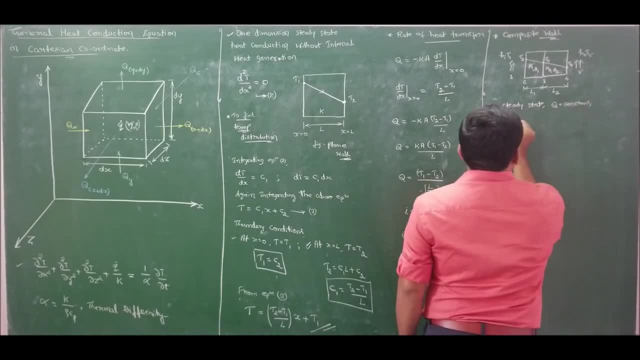 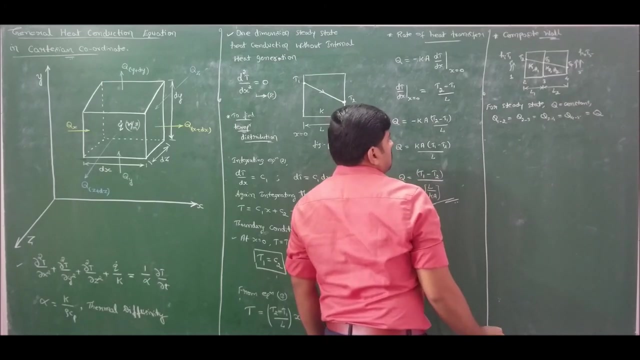 That is, q 1 to 2 is equal to q 2 to 3, is equal to q 3 to 4, which is equal to q 4 to 4.. 5 R- R equal to Q for steady state. So now, if I write heat transfer between 1 and 2, we know that 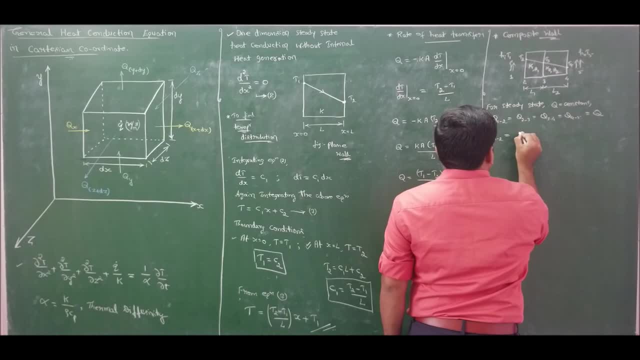 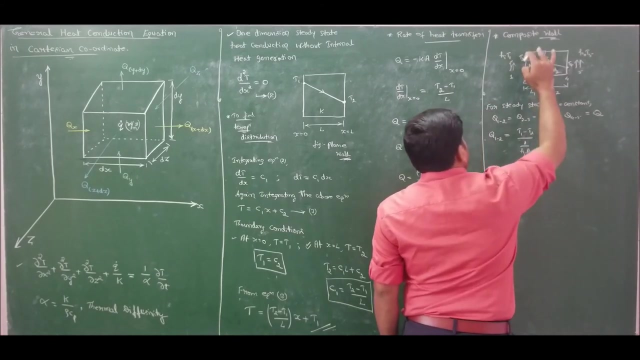 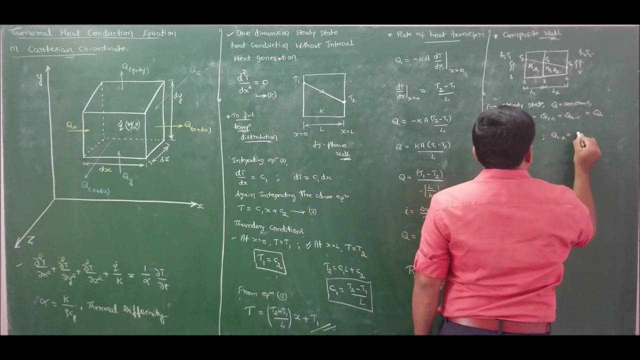 Q 1 to 2 can be written as: heat transfer due to convection, that is, temperature difference T 1 minus T 2 divided by resistance due to convection, that is 1 by H I A 1.. So this area. So therefore, I will get the value of Q 1 to 2 as or I will get the value of temperature. 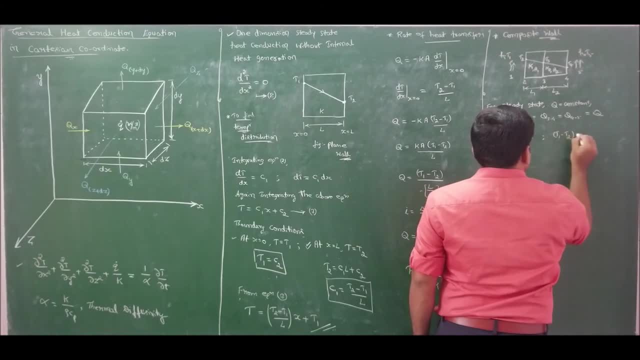 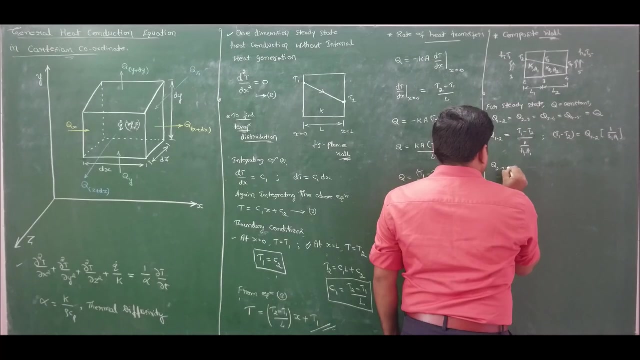 difference T 1 minus T 2 as Q 1 to 2 times 1 by H I A 1. I can call this as resistance 1. So similarly I can write for Q 2 to 3 as T 2 minus T 3.. 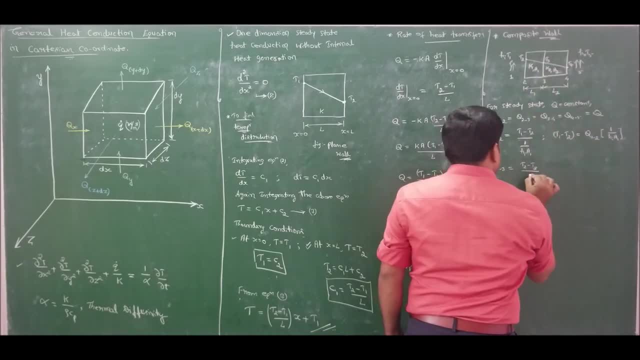 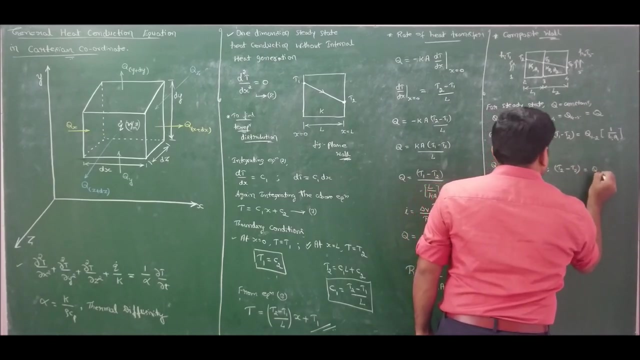 So I will get the value of T 2 minus T 3 as Q 2 to 3 times the resistance, that is, L 1 by K 1 A 1.. So hence we can write T 2 minus T 3 as Q 2 to 3 times the resistance. 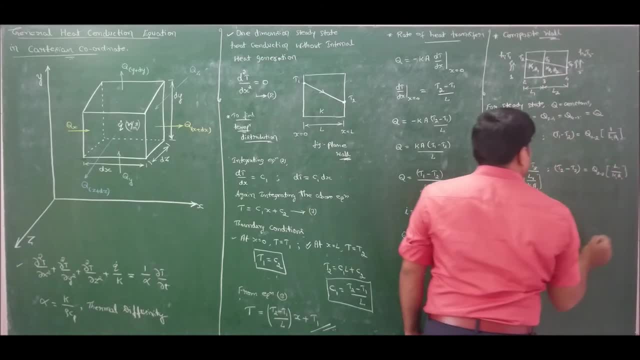 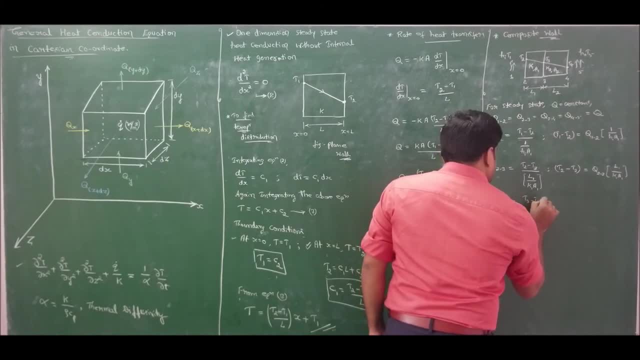 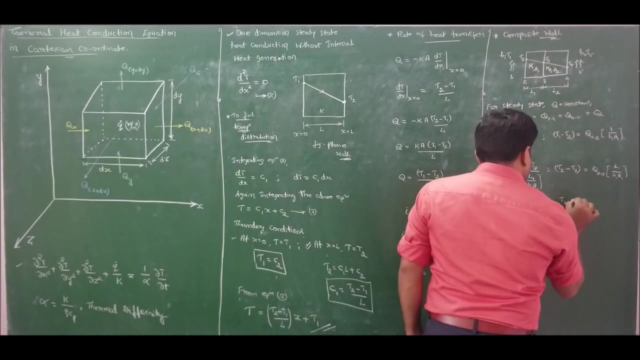 Q 3 to 4.. Again, I can write it as T3 minus T4 divided by conduction resistance, that is L2 by K2A2.. So from which we can state that T3 minus T4 is nothing but Q3Q4 times the conduction. 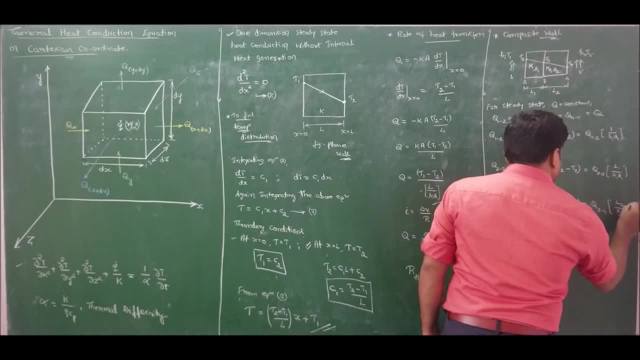 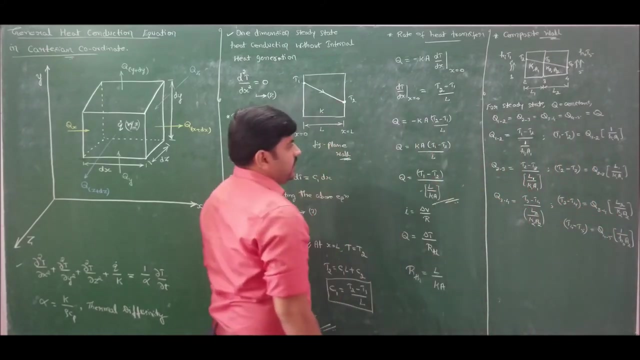 resistance: L2 by K2A2.. So similarly, I can write T4 minus T5 as Q425.. Here the resistance is because of convection, that is, 1 by H0A2.. So this is what we get. 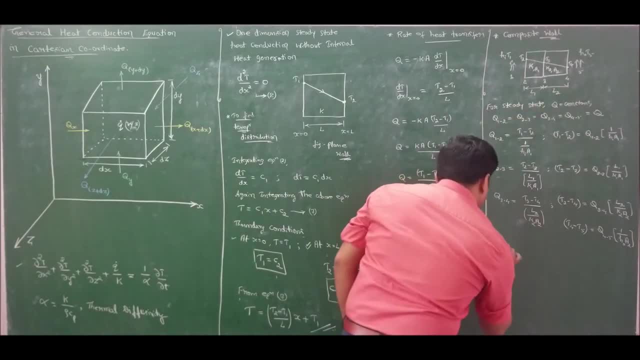 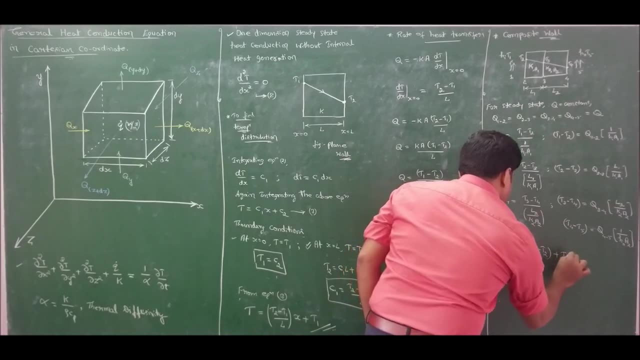 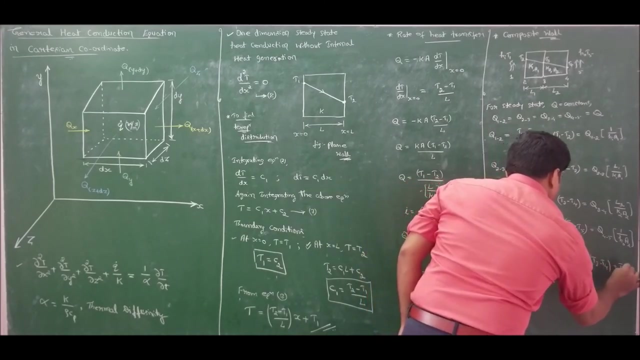 So now the temperature difference T1 minus T5 can be written as T1 minus T5, can be written as T1.. So I can write T1 minus T2 plus T2 minus T3 plus T3 minus T4 plus T4 minus T5.. 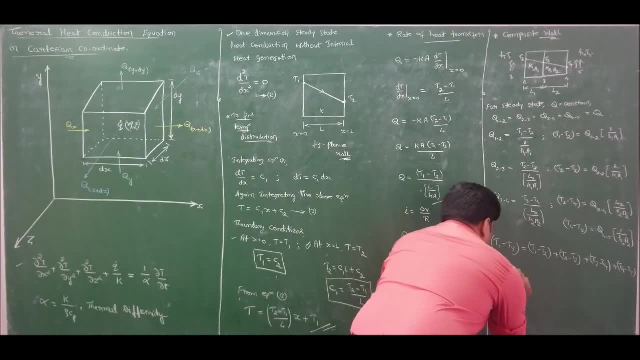 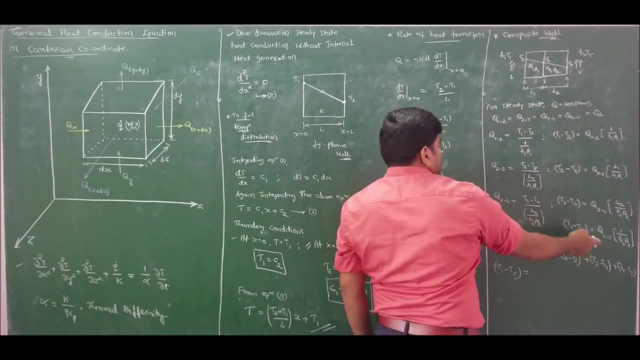 So now, if you observe, I can write T1 minus T5 as so substitute these here, and we know that the Q is constant. that is, Q12 is equal to Q23, is equal to Q34, is equal to Q45 are all equal to Q. 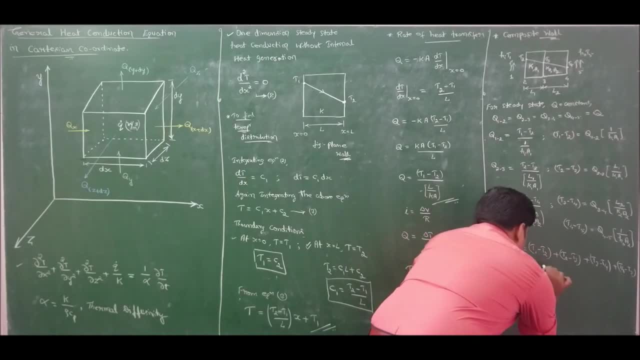 So therefore throughout, So we can take Q common. So if we take Q common, we have the resistances, that is, 1 by HIJ1 plus L1 by K1A1 plus L2 by K2A2 plus 1 by H0A2.. 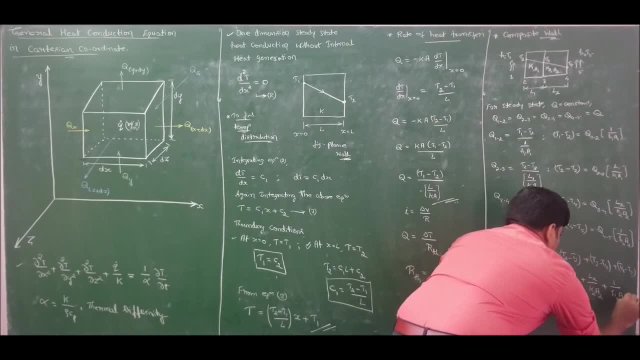 So hence I can write this as Q is equal to T1 minus T5 by sum of resistances Q. So this is equal to T1 minus T5 plus T5 minus T5 minus T5 by K2A. So now I can take: Q common plus Q is equal to T5 minus T5, and T5 minus T5 is equal to: 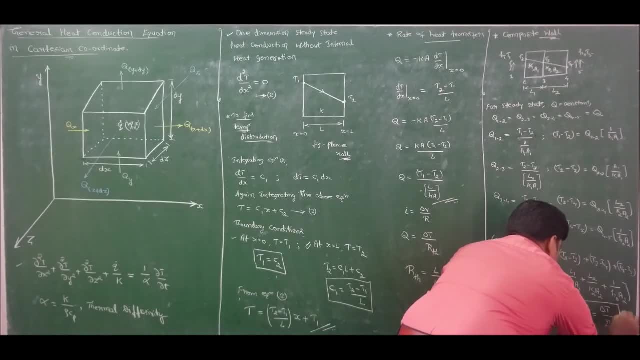 Q. So this is equal to Q by Q. So I can write Q common as Q1 minus T5 by K2.. So R1 minus T5 plus R2 plus R3 plus R4. The four resistances. so in general we can write it as: Q is equal to delta T by summation. 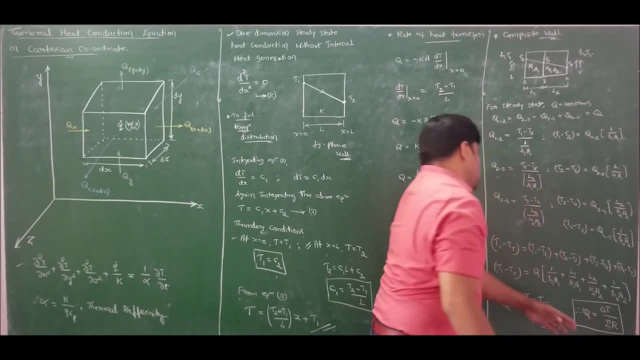 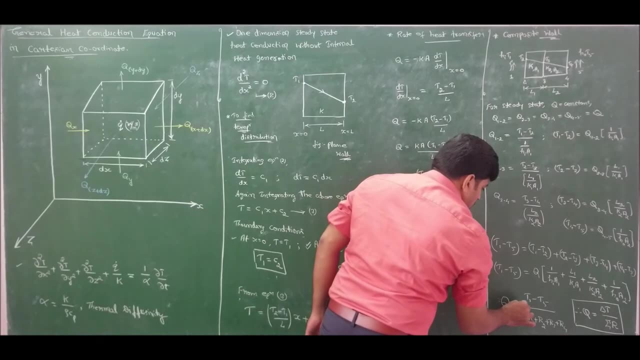 of resistances, That is, resistance to convection and conduction resistances. So this is the general expression for heat transfer through a composite wall: heat transfer through a composite wall- Right Correct Right, where R1 corresponds to 1 by H1A1,, R2 corresponds to L1 by K1A1, R3 corresponds to L2 by K2A2. 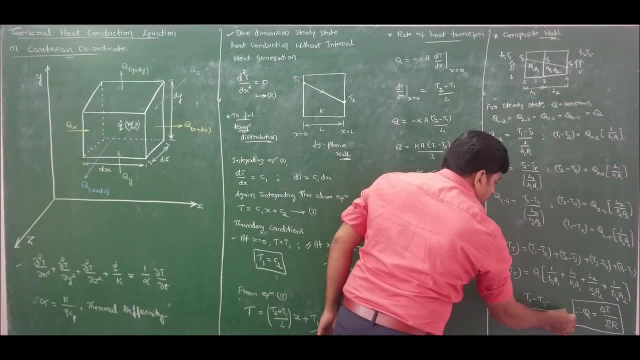 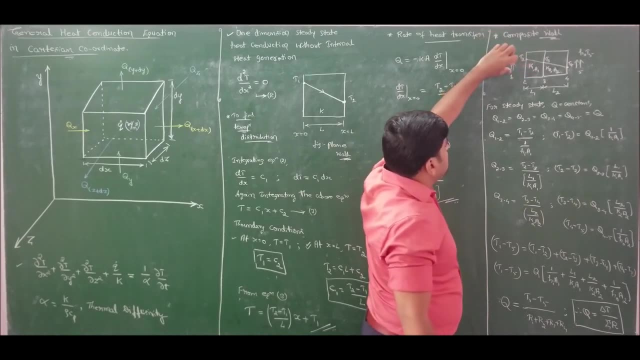 and R4 corresponds to 1 by H0A2.. And also I can write this as: if I want to write the heat transfer between 1 and 3, I can write: as: Q is equal to T1 minus T3 divided by we. 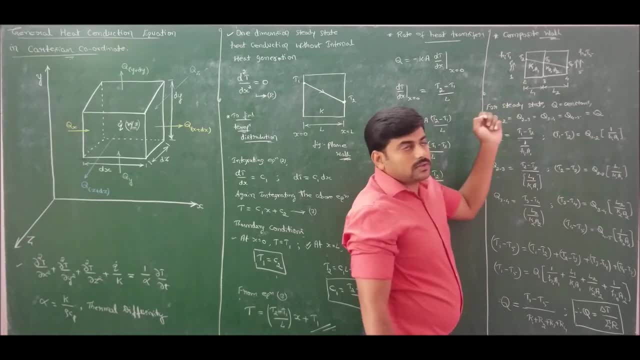 have two resistances, that is, 1 to 2 and 2 to 3, it is R1 plus R2.. Similarly, if I want to write between 2 and 4, I can write it as T2 minus T4, divided by R2 plus R3.. Similarly. 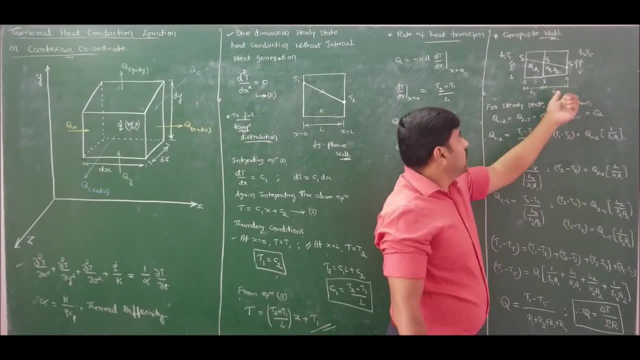 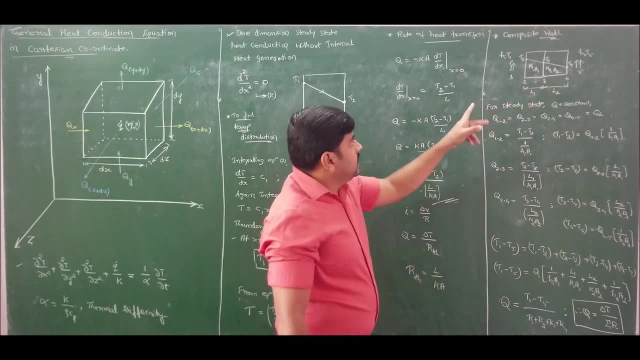 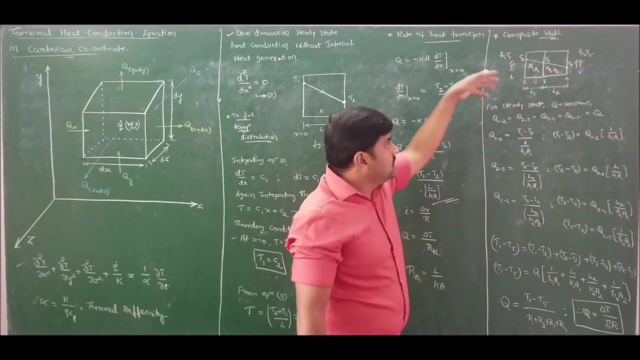 if I want to write between 3 and 5, it is T3 minus T5 divided by R3 plus R4. So you can write between any two points. It need not be consecutive. it can be a jumping of one unknown temperature in between. So this helps us to solve various types of problems. 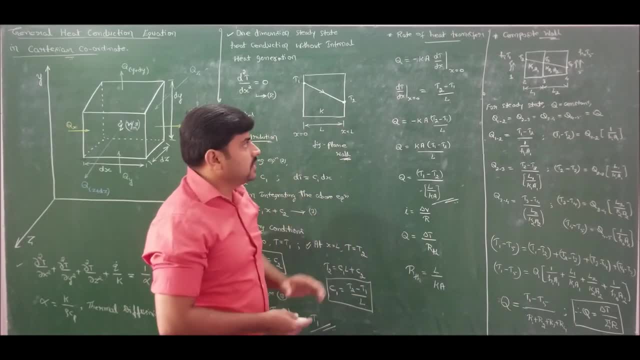 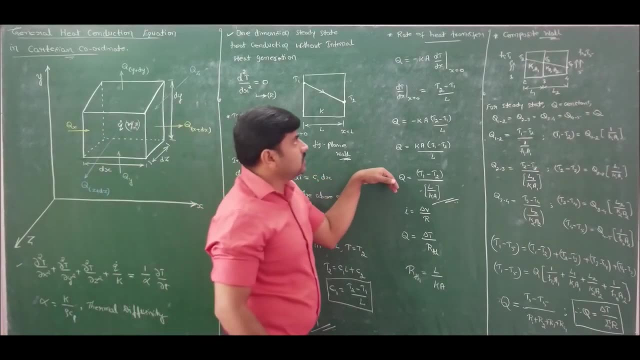 on compounds Composite walls. Once I take up problems, this will become more clear. So this is a derivation for temperature distribution and rate of heat transfer through a plane wall and also the rate of heat transfer for composite wall. That is all from this lecture. Thank.